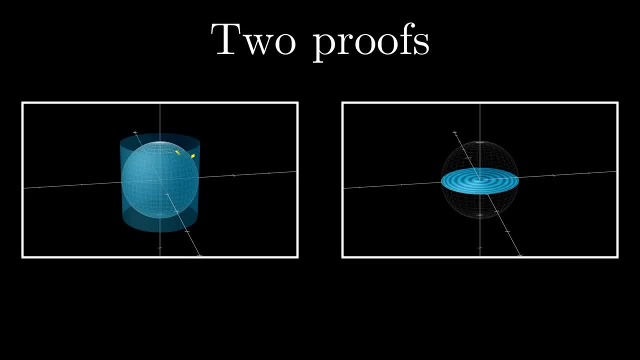 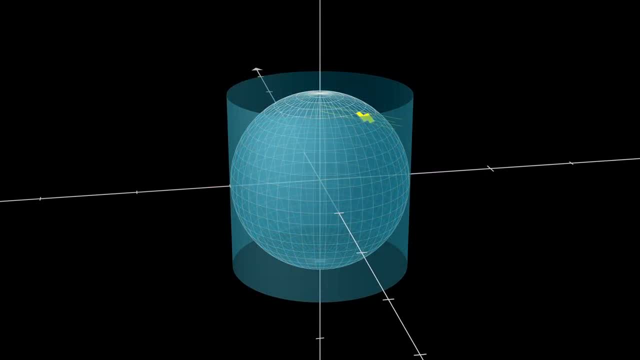 you two separate ways of thinking about the surface area that connect it in a satisfying way to these circles. The first comes from a classic, one of the true gems of geometry that I think all math students should experience the same way. all English students should read at least some Shakespeare. The second line of reasoning 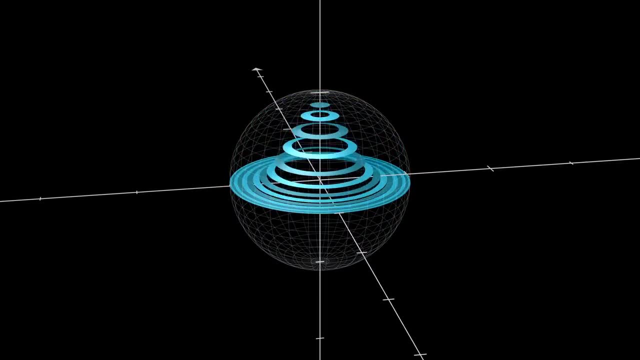 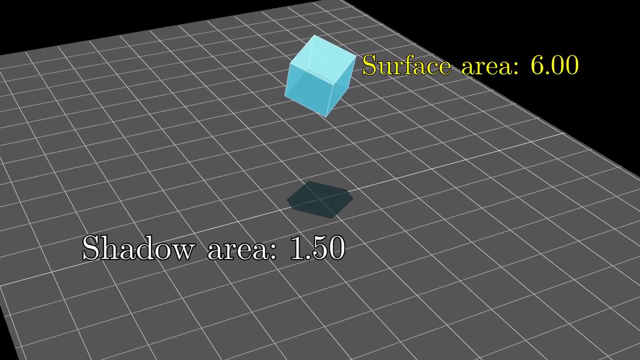 is something of my own which draws a more direct line between the sphere and its shadow. And lastly, I'll share why this fourfold relation is not unique to spheres, but is instead one specific instance of a much more general fact for all, convex shapes in three dimensions. 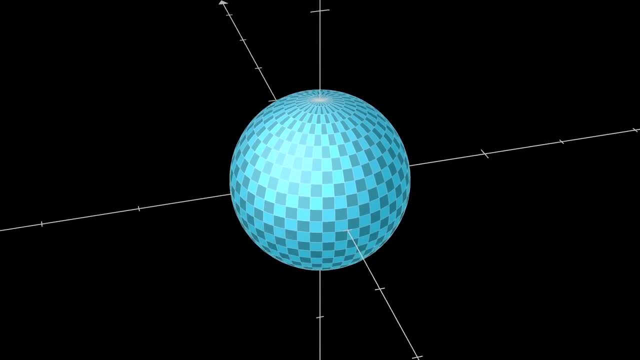 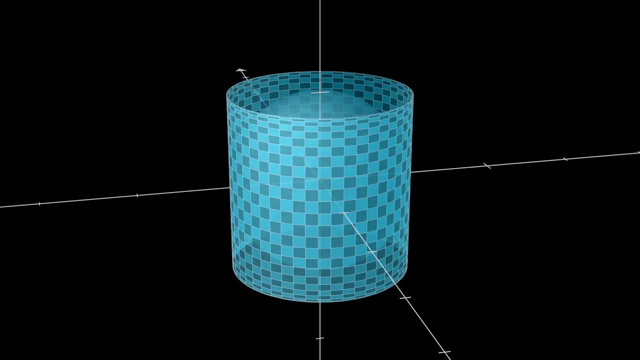 Starting with the bird's eye view here. the idea for the first approach is to show that the surface area of the sphere is the same as the area of a cylinder with the same radius and the same height as that sphere, Or rather a cylinder without the top and the bottom, what you might call the label. 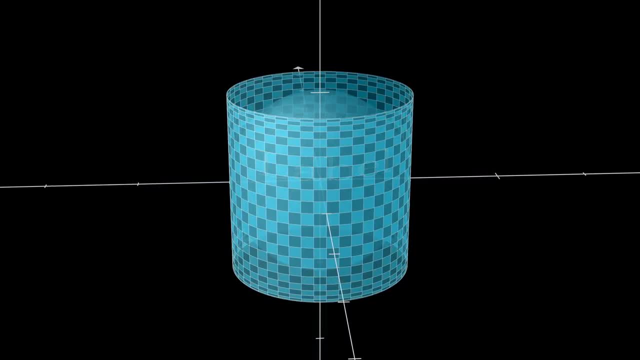 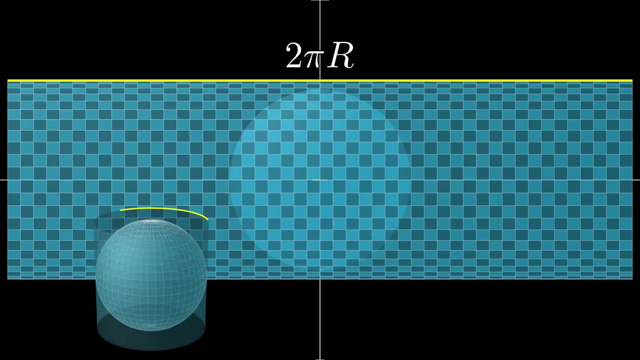 of that cylinder And once you have that, you can unwrap that label to understand it simply as a rectangle. The width of this rectangle comes from the cylinder's circumference, so it's 2 pi times r, And the height comes from the height of the sphere, which is 2 times the radius. 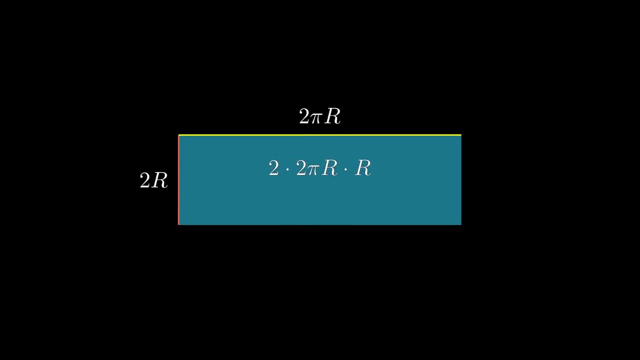 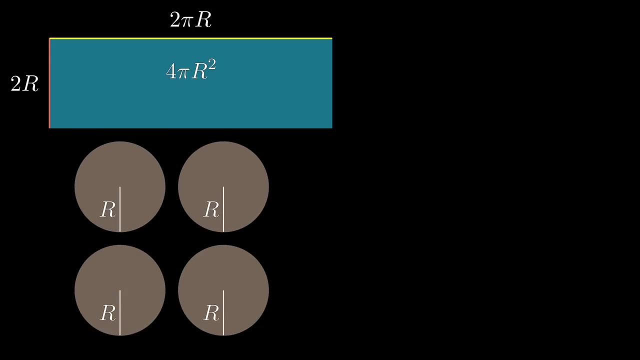 And this already gives us the formula 4 pi, r squared when we multiply the two. But in the spirit of mathematical playfulness, it's nice to see how four circles with radius r can actually fit into this picture. The idea will be to unwrap each circle into a triangle. 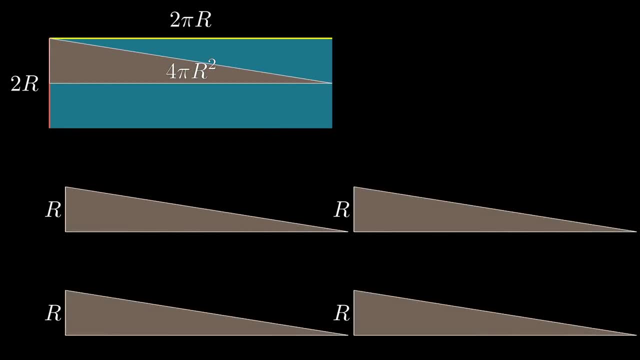 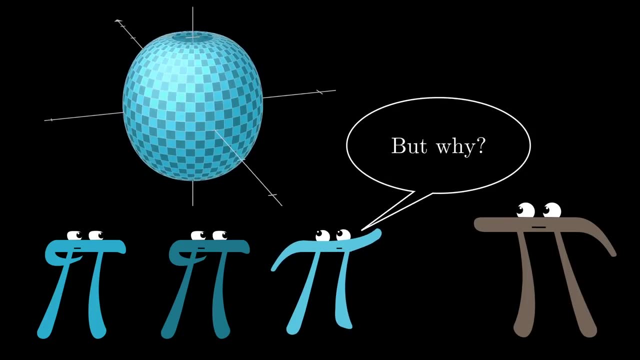 without changing its area, and then to fit those nicely into the unfolded cylinder label. More on that in a couple minutes. The more pressing question is why on earth should the sphere be related to the cylinder in this way? The way I'm animating it is already suggestive of how this might work. 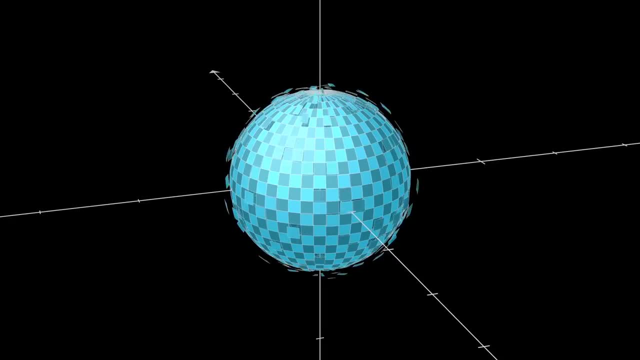 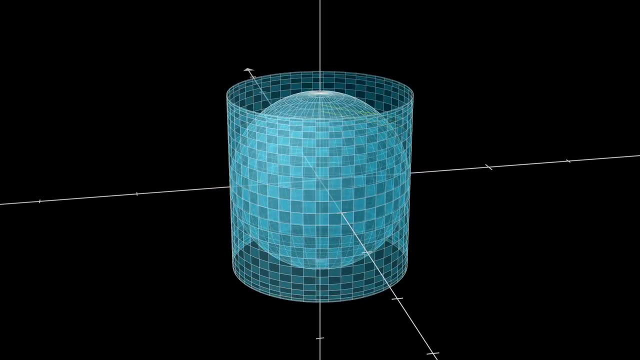 The idea is to approximate the area of the sphere with many, many tiny rectangles covering it and to show how, if you project these rectangles directly outward, as if casting a shadow, by little lights positioned on the z-axis pointing parallel to the xy-plane. 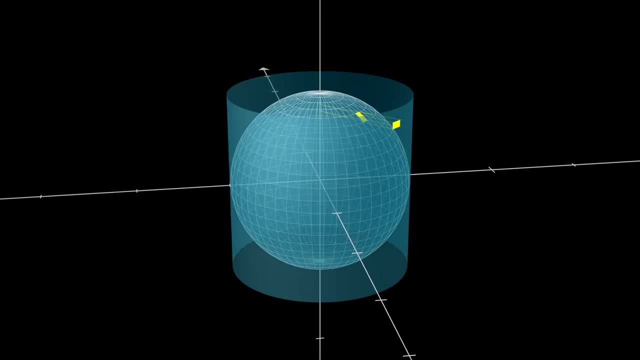 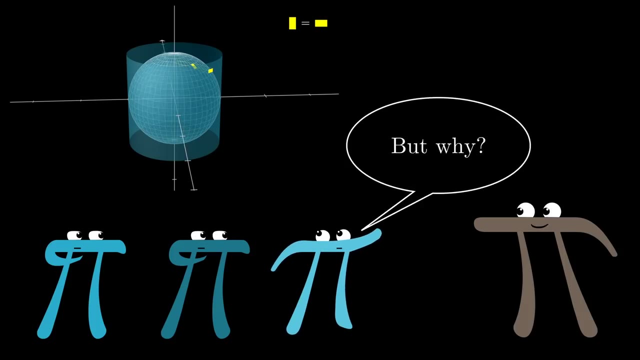 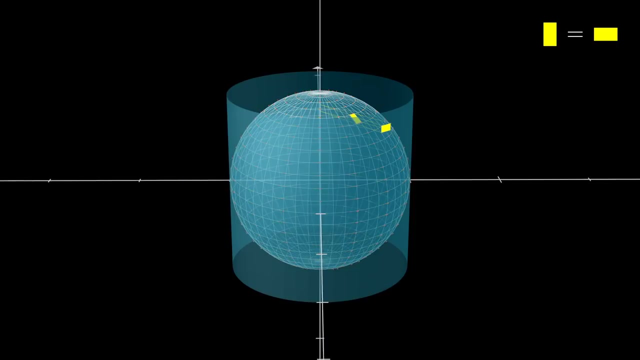 the projection of each rectangle onto the cylinder quite surprisingly ends up having a the same area as the original rectangle. But why should that be? Well, there are two competing effects at play here. For one of these rectangles, let's call the side along the latitude lines its width. 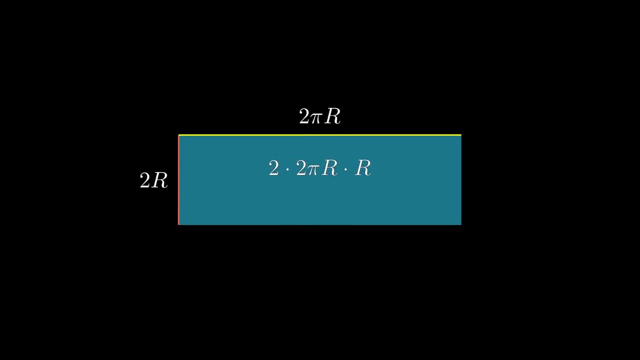 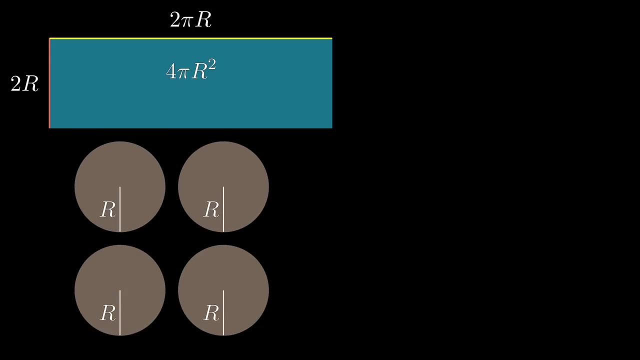 And this already gives us the formula 4 pi, r squared when we multiply the two. But in the spirit of mathematical playfulness, it's nice to see how four circles with radius r can actually fit into this picture. The idea will be to unwrap each circle into a triangle. 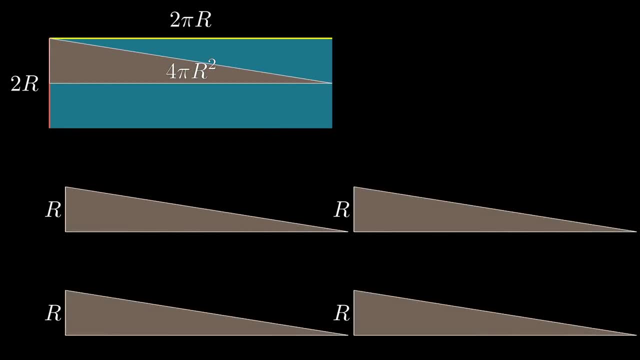 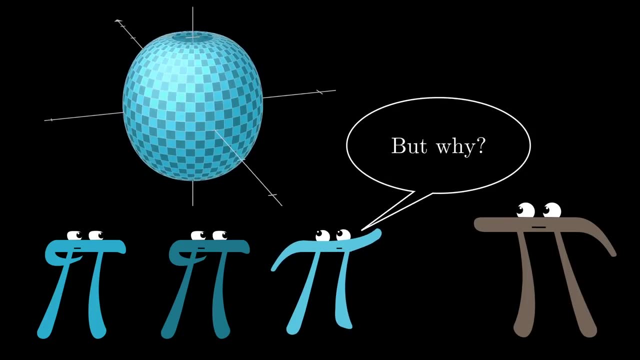 without changing its area, and then to fit those nicely into the unfolded cylinder label. More on that in a couple minutes. The more pressing question is why on earth should the sphere be related to the cylinder in this way? The way I'm animating it is already suggestive of how this might work. 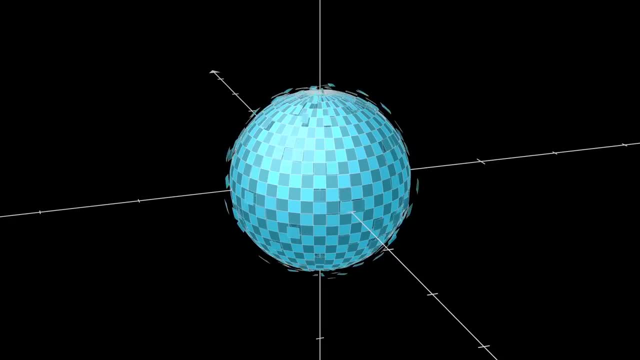 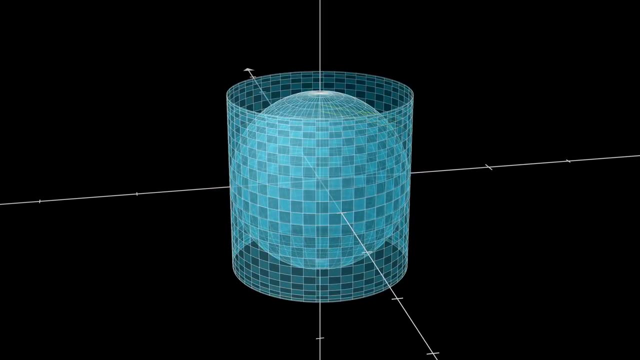 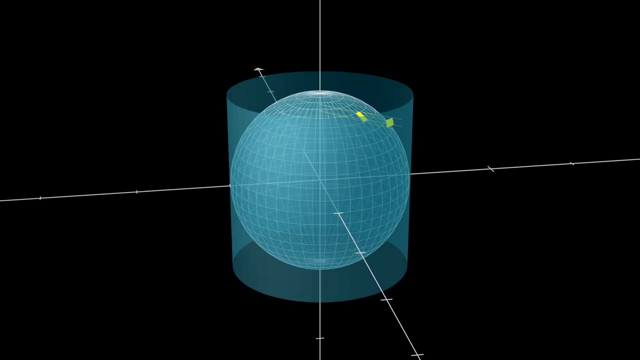 The idea is to approximate the area of the sphere with many, many tiny rectangles covering it and to show how, if you project these rectangles directly outward, as if casting a shadow, by little lights positioned on the z-axis pointing parallel to the xy-plane, the projection of each rectangle onto the cylinder quite surprisingly ends up having a 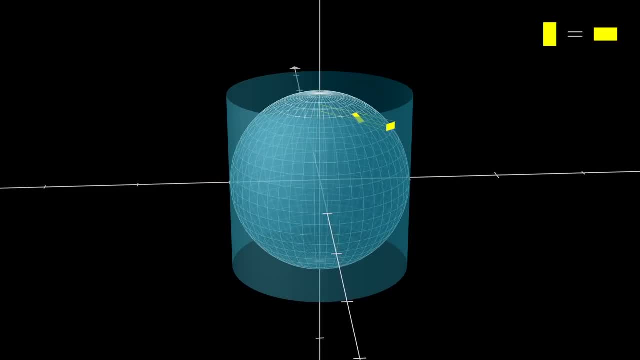 the same area as the original rectangle. But why should that be? Well, there are two competing effects at play here. For one of these rectangles, let's call the side along the latitude lines its width, and the side along the longitude lines, its height. On the one hand, as the rectangle is projected outward, its width will get scaled up. For rectangles towards the poles, that length is scaled up quite a bit, since they're projected over a longer distance, But for those closer to the equator the effect might be close to nothing. 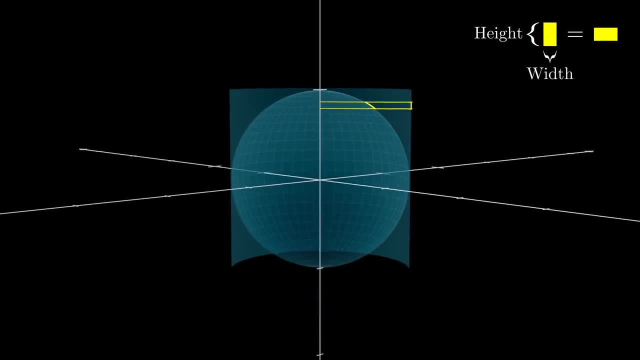 But, on the other hand, because these rectangles are already slant with respect to the z-direction, during this projection, the height of each such rectangle will get scaled down. Think about holding some flat object and looking at its shadow As you reorient that object. 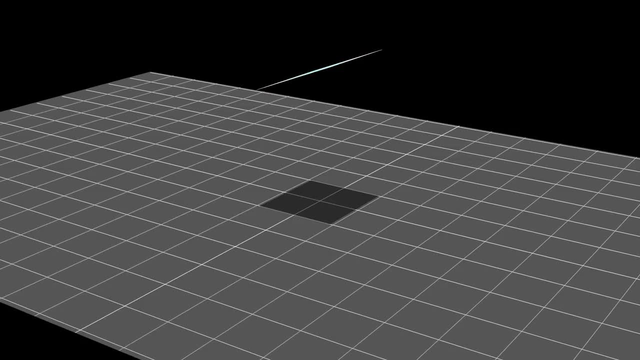 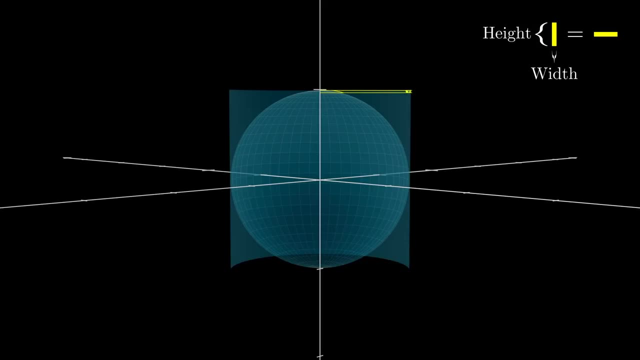 the shadow looks more or less squished for some angles. Now take a look: Those rectangles towards the poles are quite slanted this way, so their height is going to get squished down by a lot. For those closer to the equator, oriented somewhere closer to parallel to the z-axis, 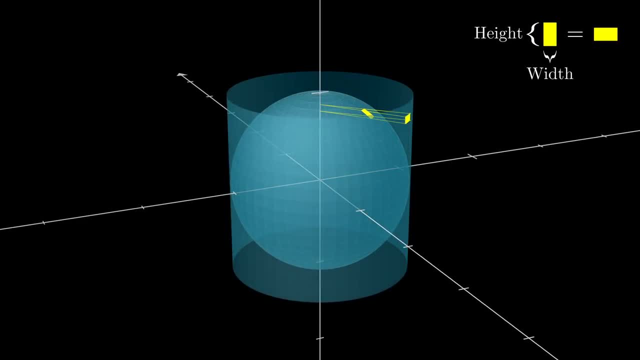 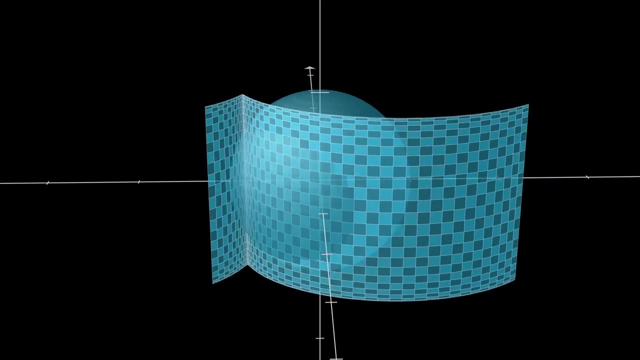 the effect is not as much. It will turn out that these two effects of stretching the width and squishing the height cancel each other out perfectly Already as a rough sketch. wouldn't you agree that this is a very pretty way of reasoning? 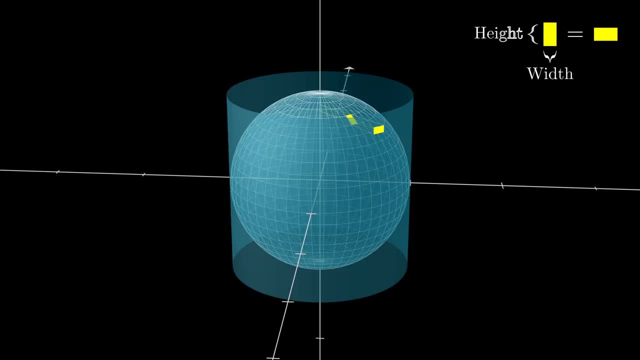 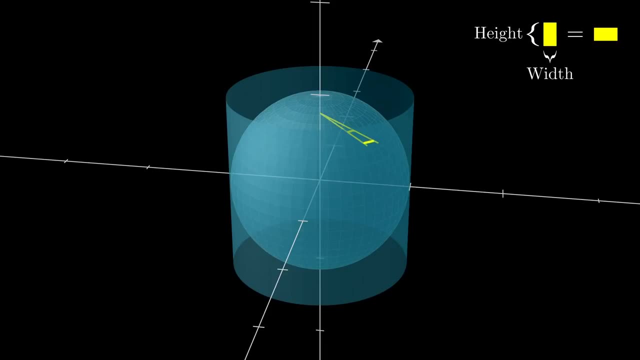 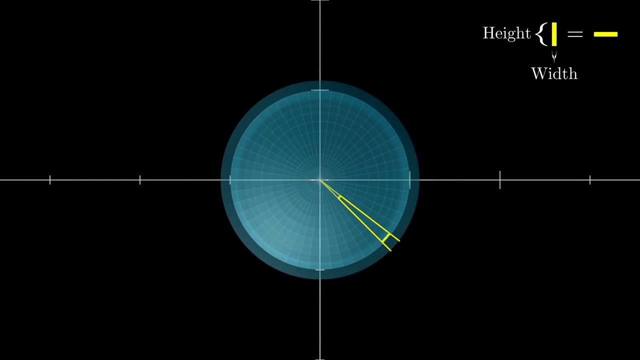 and the side along the longitude lines, its height. On the one hand, as the rectangle is projected outward, its width will get scaled up. For rectangles towards the poles that length is scaled up quite a bit since they're projected over a longer distance. But for those closer to the equator the effect might be close to nothing. 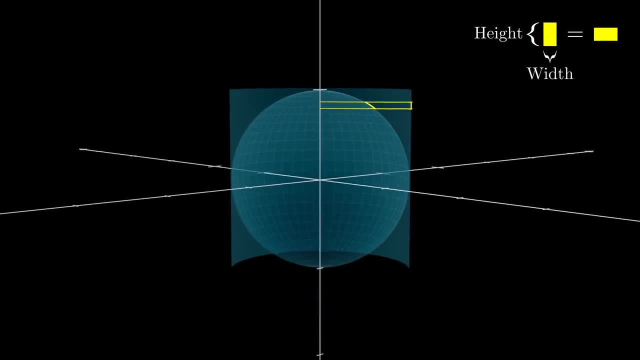 But, on the other hand, because these rectangles are already slant with respect to the z-direction, during this projection, the height of each such rectangle will get scaled down. Think about holding some flat object and looking at its shadow As you reorient that object. 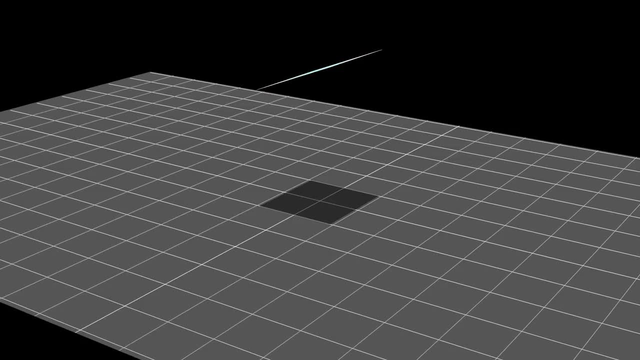 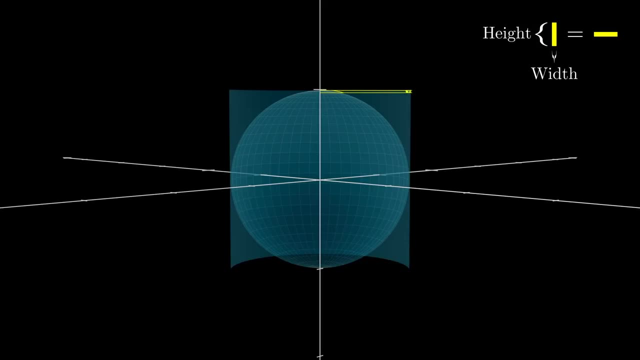 the shadow looks more or less squished for some angles. Now take a look: Those rectangles towards the poles are quite slanted this way, so their height is going to get squished down by a lot. For those closer to the equator, oriented somewhere closer to parallel to the z-axis, 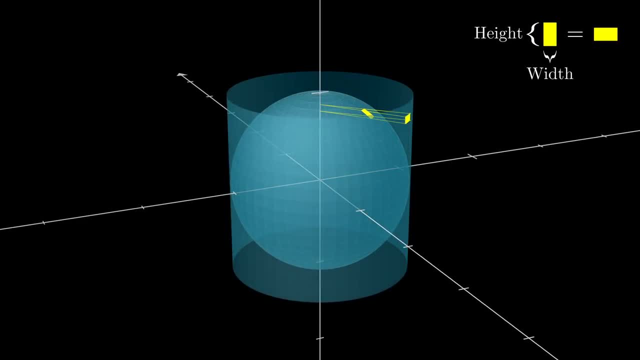 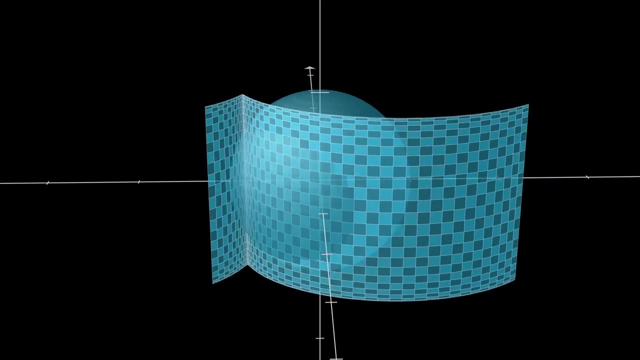 the effect is not as much. It will turn out that these two effects of stretching the width and squishing the height cancel each other out perfectly Already as a rough sketch. wouldn't you agree that this is a very pretty way of reasoning? 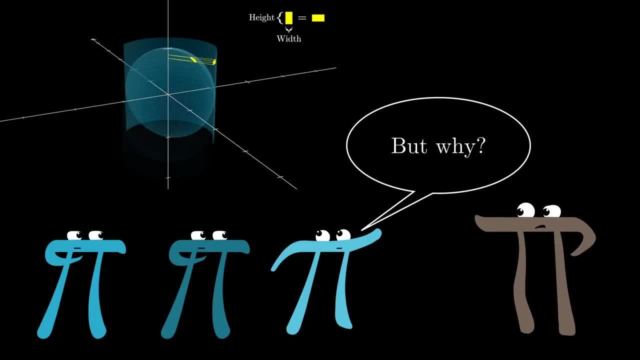 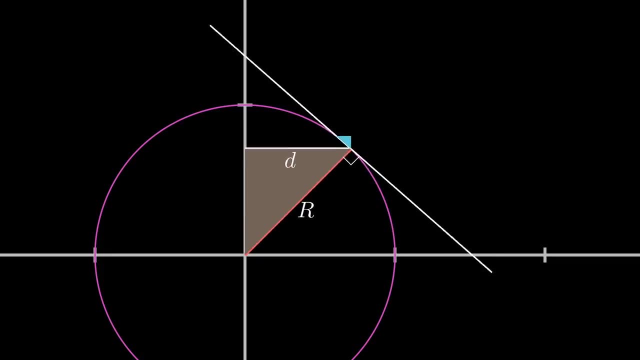 Of course, the meat here comes from showing why these two competing effects can in some ways cancel each other out, And in some ways, the details fleshing this out are just as pretty as the zoomed-out structure of the full argument. 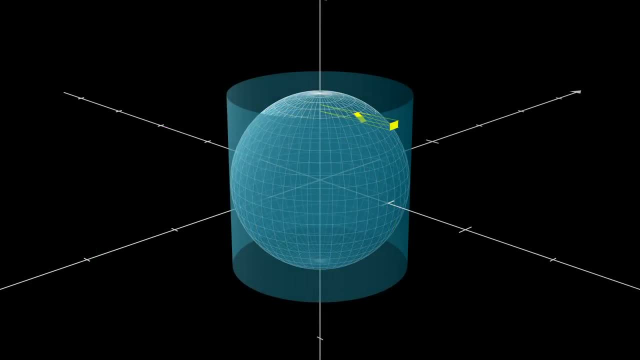 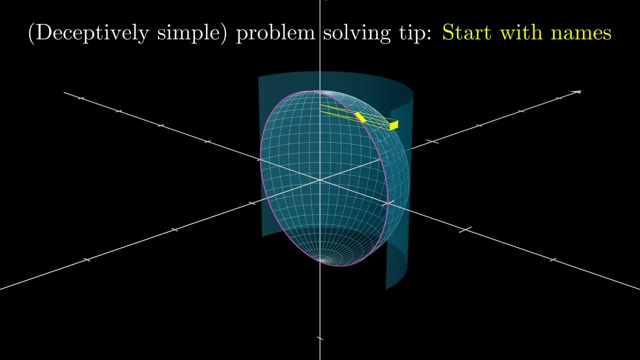 So let's dig in. Let me go ahead and cut away half of the sphere so that we can get a better look For any mathematical problem solving. it never hurts to start by giving things names. So let's say that the radius of the sphere is r. 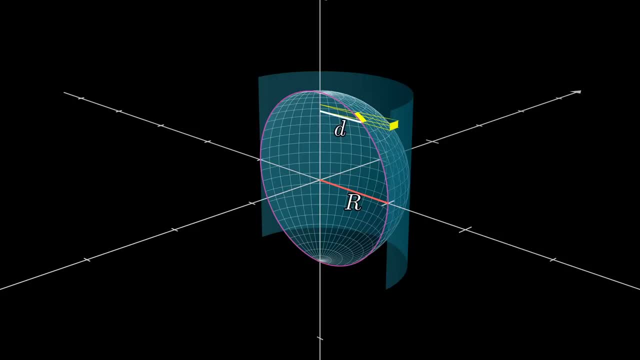 and for one specific rectangle, let's call the distance between that rectangle and the z-axis d. So let's say that the radius of the sphere is r, and for one specific rectangle, let's call the distance between that rectangle and the z-axis d. 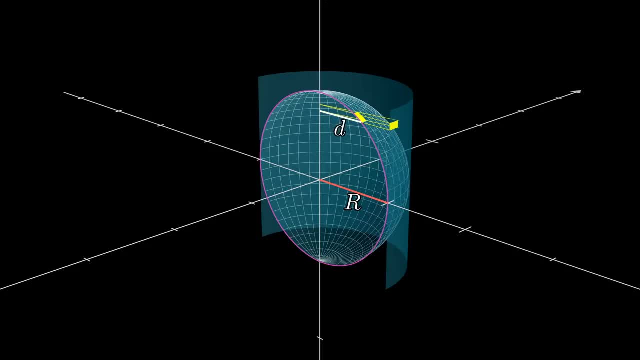 You really want to know what the radius of the sphere is, and you can do that by looking at the rectangle. You could rightfully complain that the distance d is a little ambiguous depending on which point of that rectangle you're going from, But for tinier and tinier rectangles that ambiguity will become negligible. 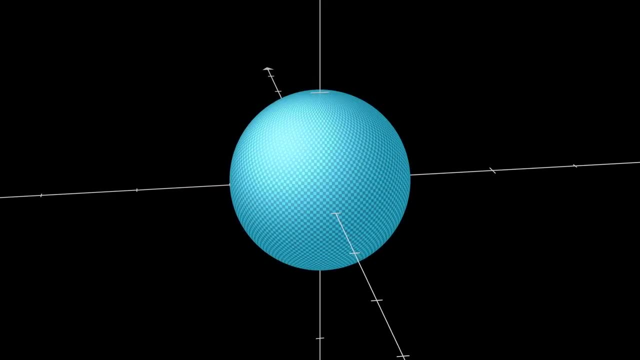 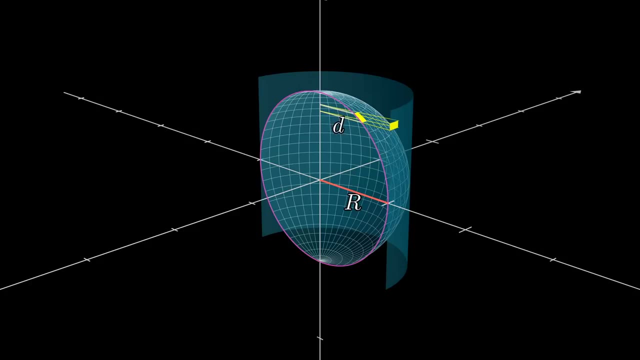 And tinier and tinier is when this approximation with rectangles gets closer to the true surface area. anyway, To choose an arbitrary standard, let's say that d is the distance from the bottom of the rectangle. Now to think about projecting this out to the cylinder. 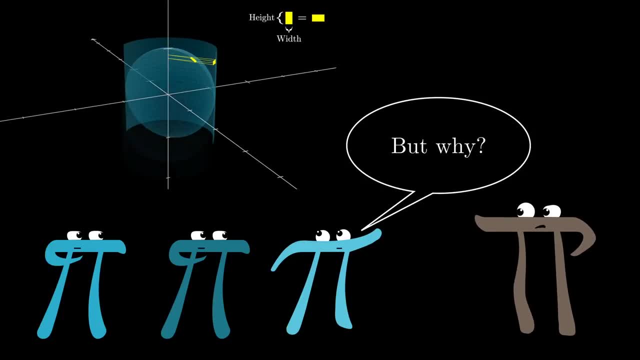 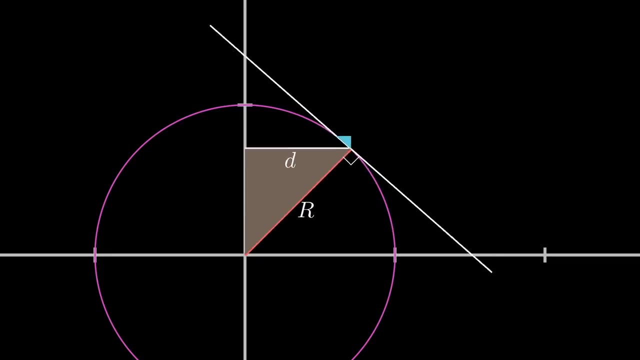 Of course, the meat here comes from showing why these two competing effects can in fact cancel each other out. And in some ways, the details fleshing this out are just as pretty as the zoomed out structure of the full argument. So let's dig in. 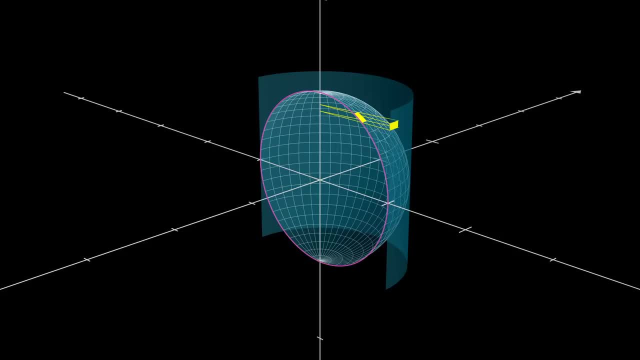 Let me go ahead and cut away half of the sphere so we can get a better look For any mathematical problem solving. it never hurts to start by giving things names. So let's say the radius of the sphere is r and for one specific rectangle, 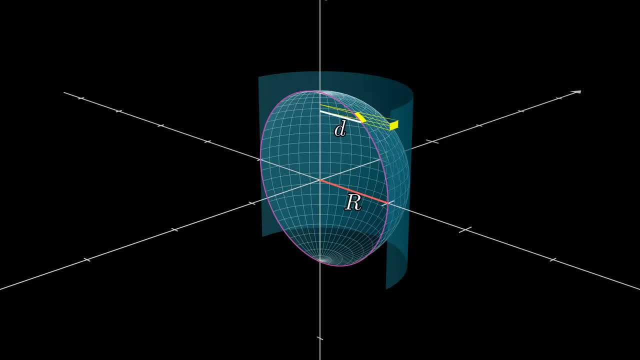 let's call the distance between that rectangle and the z-axis d. R is the radius of the sphere and for one specific rectangle, let's call the distance between that rectangle and the z-axis d. Let's call the distance between that rectangle and the z-axis d. 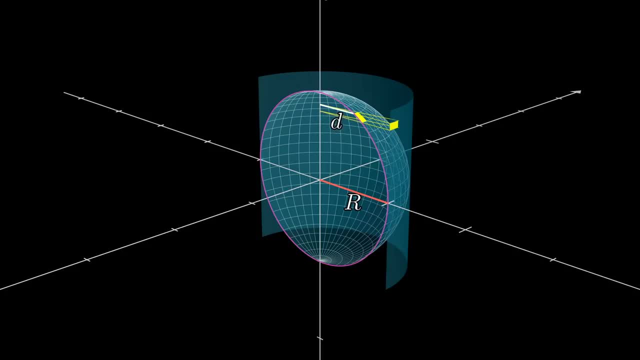 You could rightfully complain that the distance d is a little ambiguous depending on which point of that rectangle you're going from. But for tinier and tinier rectangles that ambiguity will become negligible, And tinier and tinier is when this approximation with rectangles 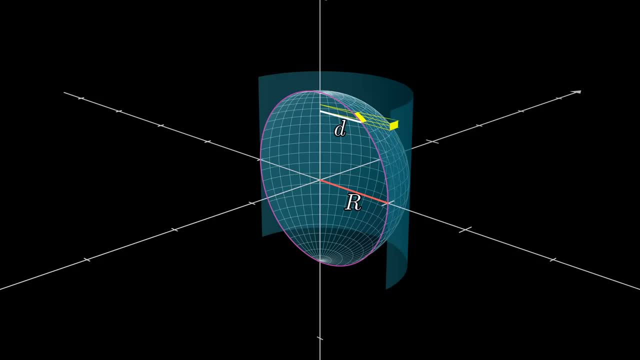 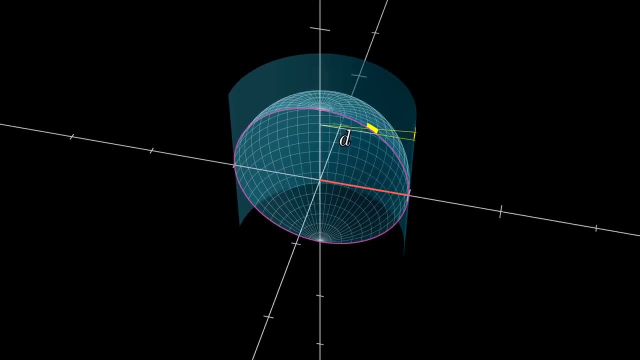 gets closer to the true surface area. anyway, To choose an arbitrary standard, let's say that d is the distance from the bottom of the rectangle. Now to think about projecting this out to the cylinder, what we're going to do is picture two similar triangles. 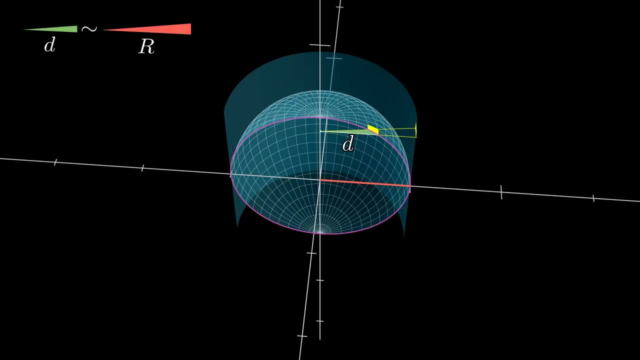 The first one shares its base with the base of the rectangle on the sphere and has a tip at the same height, but on the z-axis a distance d away. The second triangle is a scaled-up version of this, scaled so that it just barely reaches the cylinder, meaning its long side now has a length r. 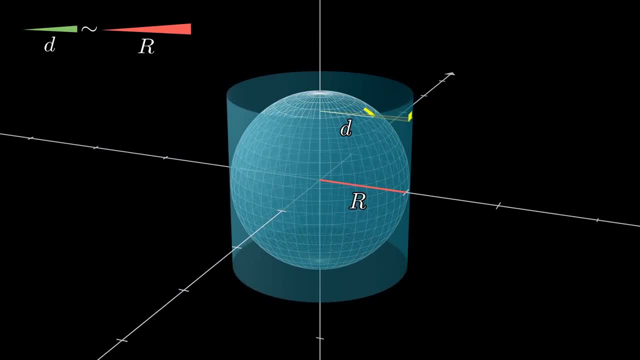 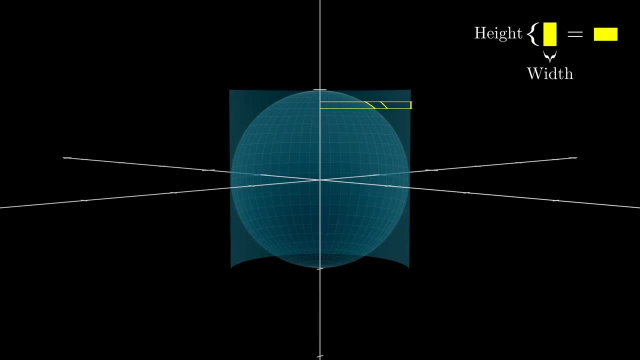 So the ratio of their bases, which is how much our rectangle's width gets stretched out, is r divided by d. What about the height? How precisely does that get scaled down as we project? Again, let's slice a cross-section for a cleaner view. 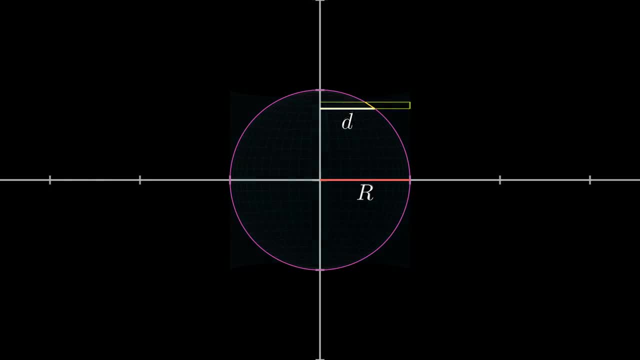 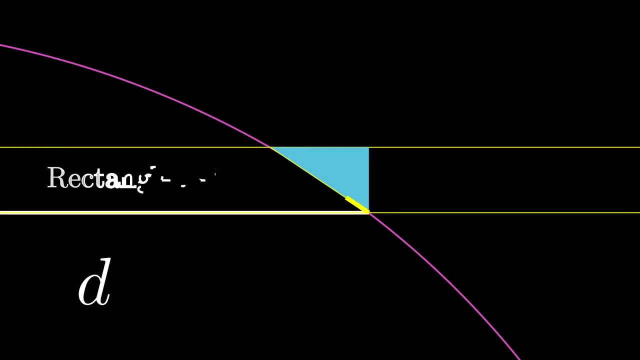 And in fact, why don't we go ahead and completely focus our view to this two-dimensional cross-section? To think about the projection, let's make a little right triangle like this, where what was the height of our spherical rectangle is the hypotenuse. 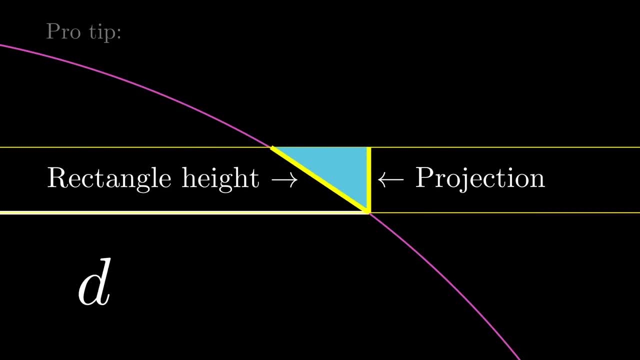 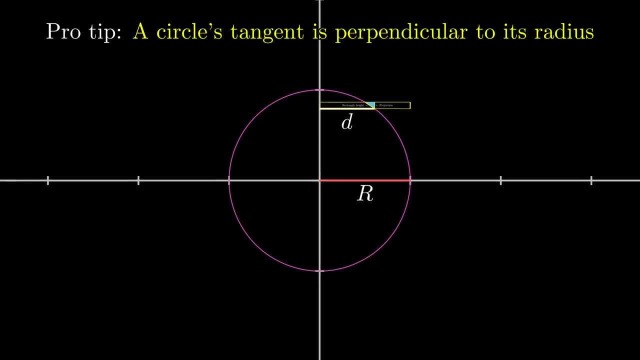 and the projection is one of the legs. Pro tip: any time you're doing geometry with circles or spheres, keep in the forefront of your mind that anything tangential is perpendicular to the radius drawn to that point of tangency. It's crazy just how helpful that one little fact can be for making progress. 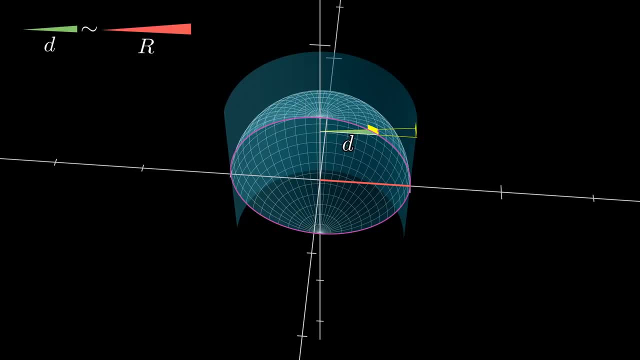 what we're going to do is picture two similar triangles. The first one shares its base with the base of the rectangle on the sphere and has a tip at the same height, but on the z-axis a distance d away. The second triangle is a scaled-up version of this. 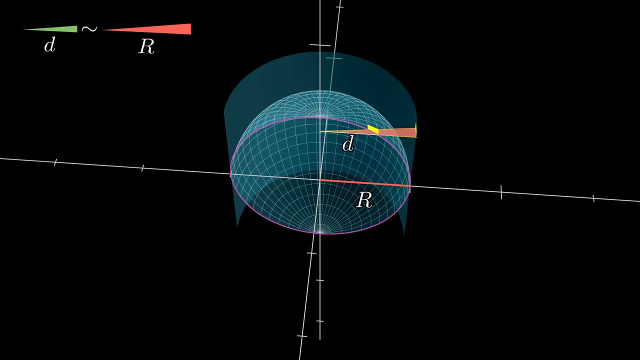 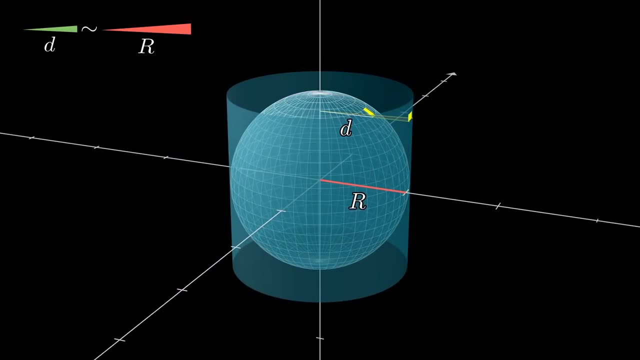 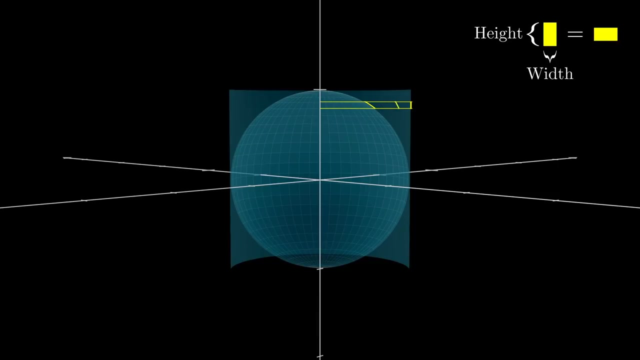 scaled so that it just barely reaches the cylinder, meaning its long side now has a length r. So the ratio of their bases, which is how much our rectangle's width gets stretched out, is r divided by d. What about the height? How precisely does that get scaled down as we project? 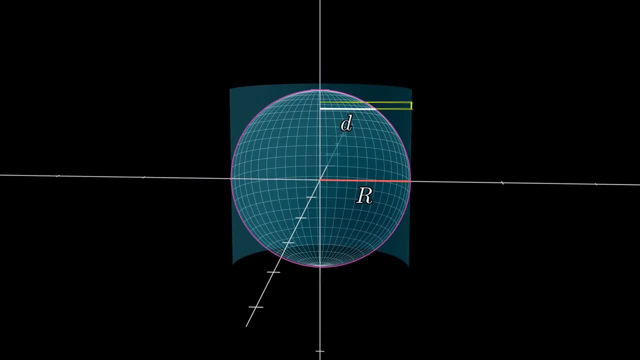 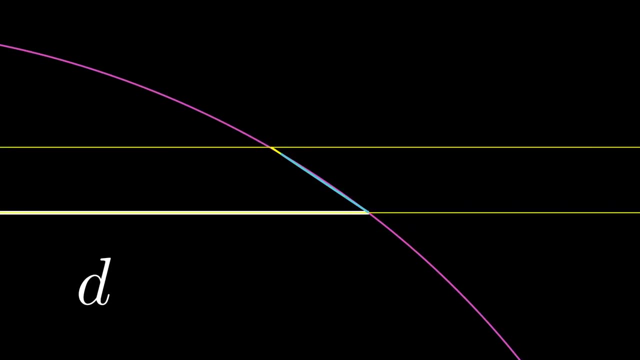 Again, let's slice a cross-section for a cleaner view And, in fact, why don't we go ahead and completely focus our view to this two-dimensional cross-section? To think about the projection, let's make a little right triangle like this: 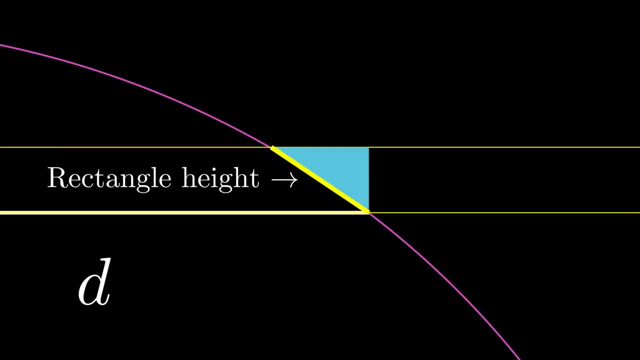 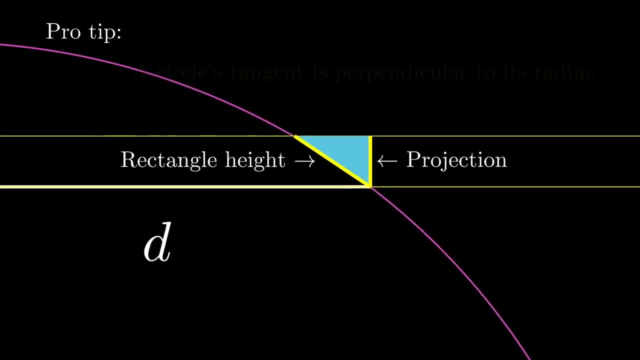 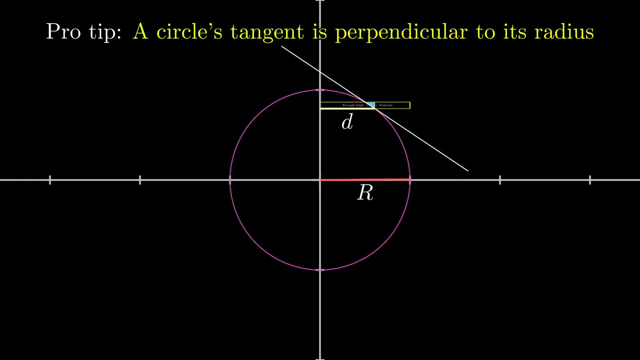 where what was the height of our spherical rectangle is the hypotenuse and the projection is one of the legs. Pro tip: any time you're doing geometry with circles or spheres, keep in the forefront of your mind that anything tangential is perpendicular to the radius drawn to that point of tangency. 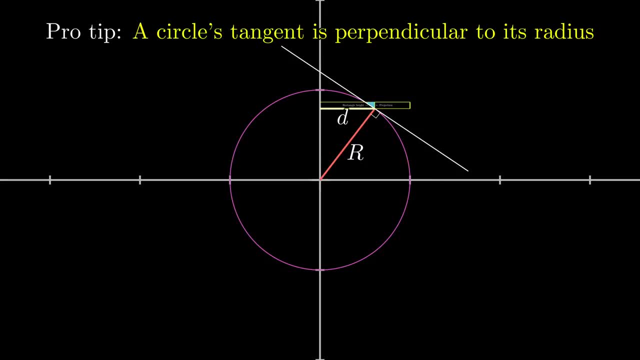 It's crazy just how helpful that one little fact can be for making progress. In our case, once we draw that radial line together with the distance d, we have another right triangle, And often in geometry, I like to imagine tweaking the parameters of a setup. 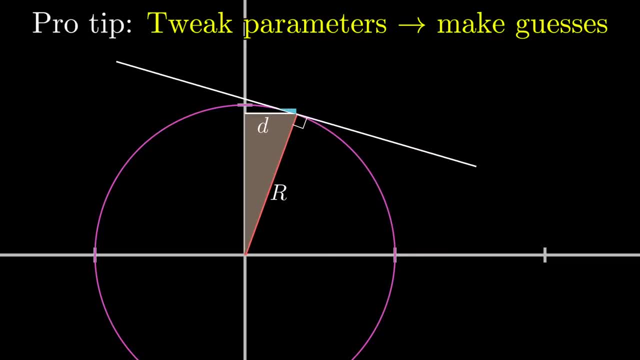 and imagining how the relevant shapes change. This helps to make guesses about what the relations might be. In this case, you might predict that the two triangles are the same and that the angles I've drawn are similar to each other, since their shapes seem to change in concert with each other. 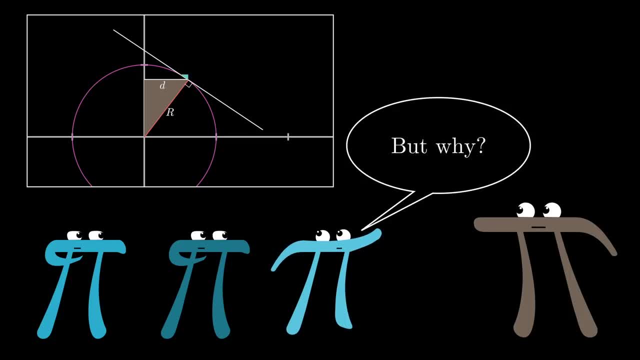 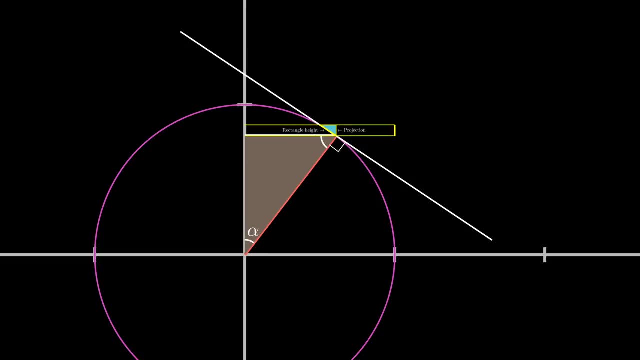 This is indeed true, but as always, don't take my word for it. See if you can justify this for yourself. Again, it never hurts to give more names to things. Maybe let's call this angle alpha and this other one beta. 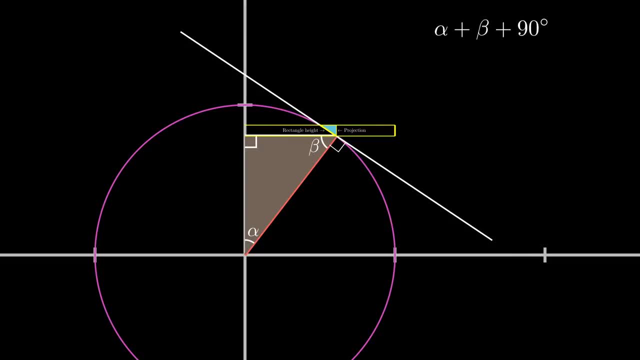 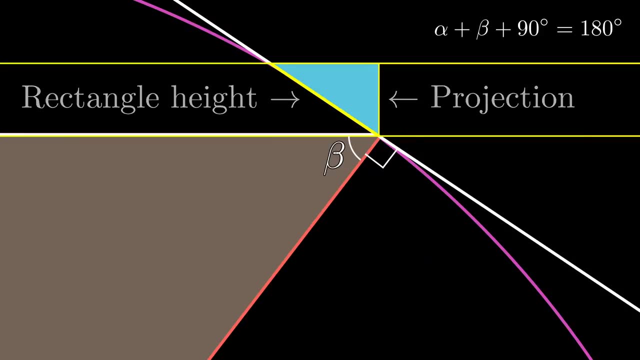 Since this is a right triangle, we know that alpha plus beta plus 90 degrees must be 180 degrees. Now let's look at this little triangle and see if we can figure out what its angles might be. Notice this 90 degree angle, which comes from the radius being perpendicular to the tangent. 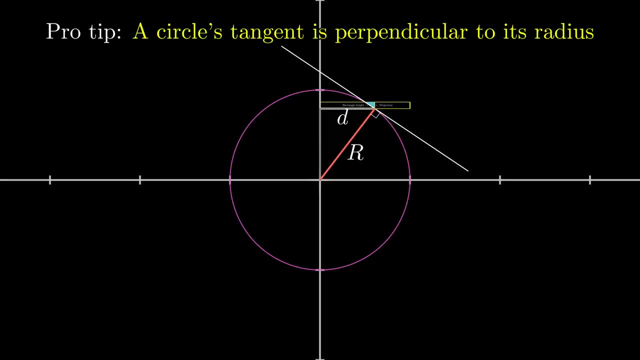 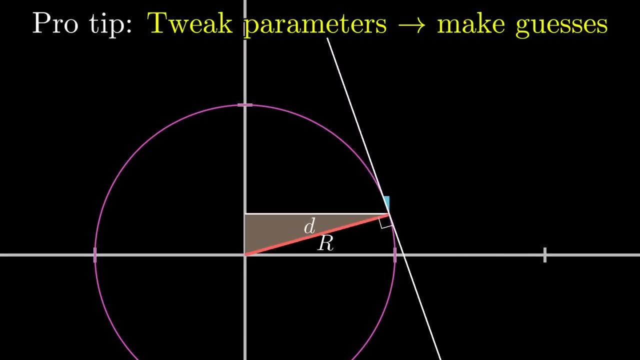 In our case, once we draw that radial line together with the distance d, we have another right triangle, And often in geometry I like to imagine tweaking the parameters of a setup and imagining how the relevant shapes change. This helps to make guesses about what the relations might be. 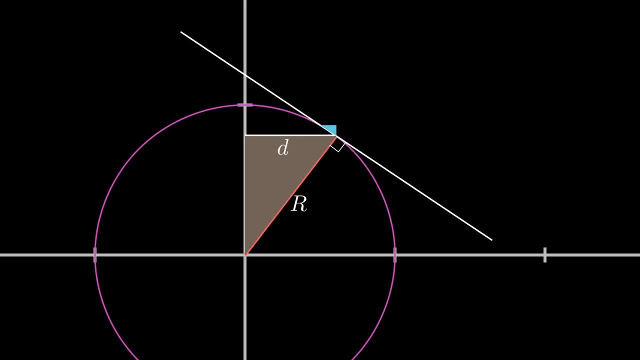 In this case, you might predict that the two triangles are the same and that the angles I've drawn are similar to each other, since their shapes seem to change in concert with each other. This is indeed true, but, as always, don't take my word for it. 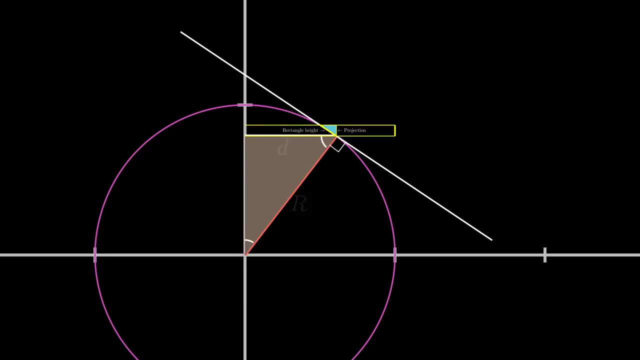 See if you can justify this for yourself. Again, it never hurts to give more names to things. Maybe let's call this angle alpha and this other one beta, Since this is a right triangle. we know that alpha plus beta plus 90 degrees must be 180 degrees. 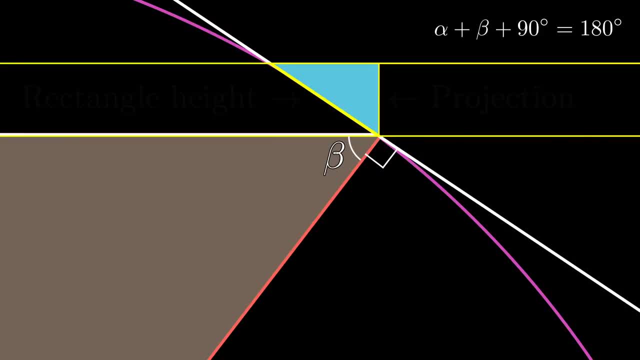 So let's look at this little triangle and see if we can figure out what its angles might be. Notice this 90 degree angle which comes from the radius being perpendicular to the tangent, and how, when it's combined with this beta here and some other little angle, it forms a straight line. 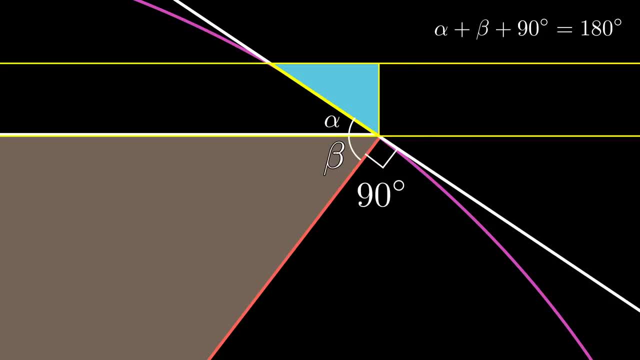 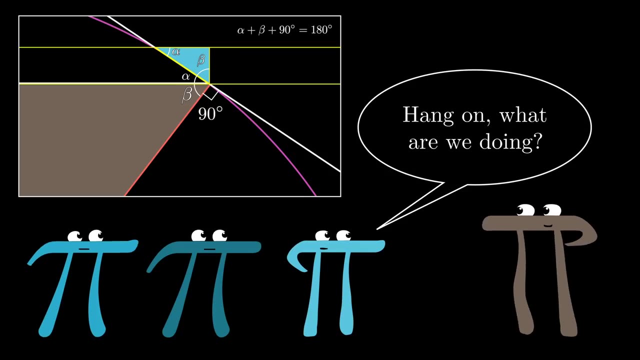 So that other little angle must be alpha, And this- lets us fill out a few more values- which reveals that this little triangle also has angles alpha, beta and 90 degrees, So it is indeed similar to the big one. Deep in the weeds like this, it's sometimes easy to forget why we're doing this. 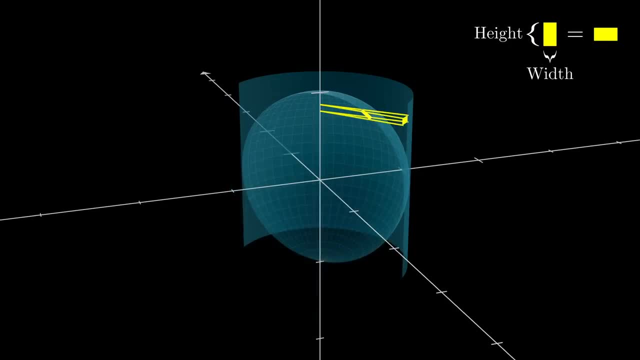 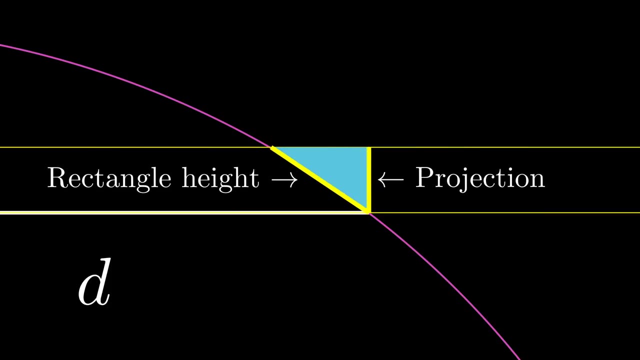 Remember. what we want to know is how much the height of the sphere rectangle gets squished down as we project it out, And that's the ratio of this little hypotenuse to the leg on the right side By the similarity with the big triangle. the ratio of those two sides is again r divided by d. 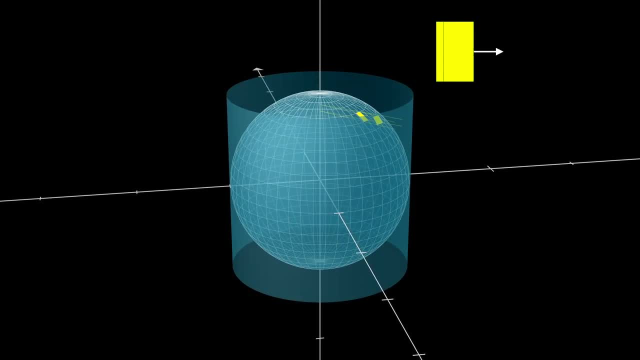 So, indeed, as this rectangle gets projected outward, the effect of stretching out the width is perfectly cancelled out by how much that height is getting squished due to the slant. As a fun side note, you might notice that it looks like the projected rectangle. 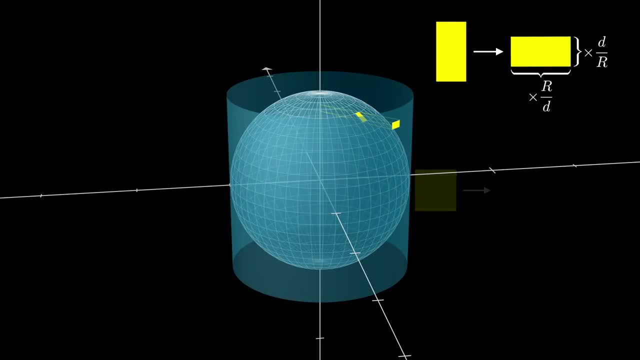 is a 90 degree rotation of the original. This would not at all be true in general, but by a lovely coincidence, the way I'm parametrizing the sphere results in rectangles where the ratio of the width to the height starts out as d to r. 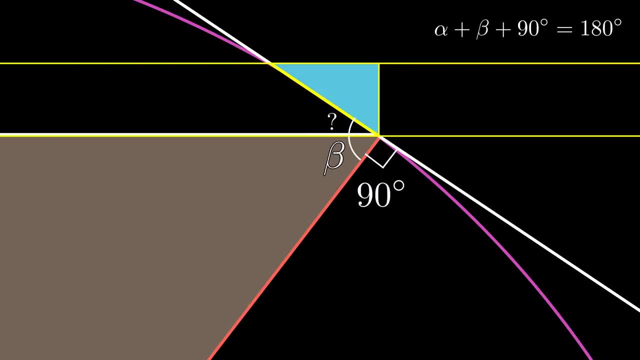 and how, when it's combined with this beta here and some other little angle, it forms a straight line, so that other little angle must be alpha And this- lets us fill out a few more values, which reveals that this little triangle also has angles alpha, beta and 90 degrees. 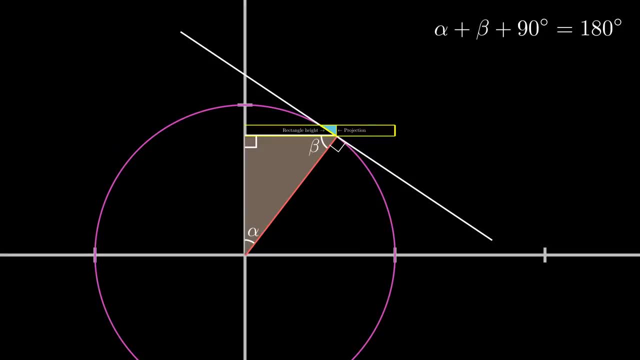 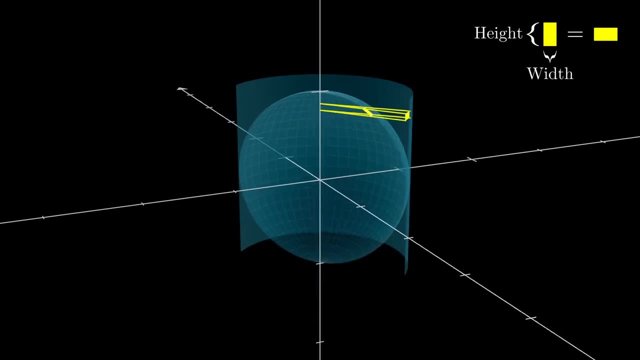 So it is indeed similar to the big one. Deep in the weeds like this, it's sometimes easy to forget why we're doing this. Remember: what we want to know is how much the height of the sphere rectangle gets squished down as we project it out. 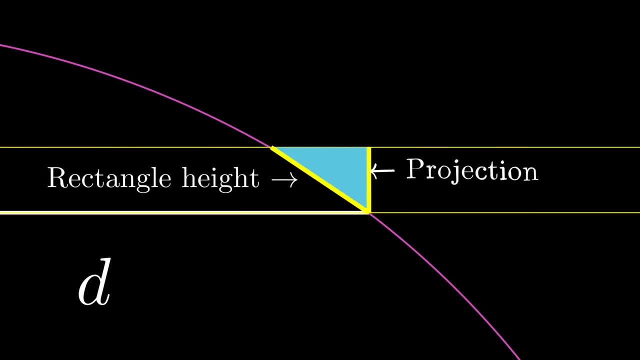 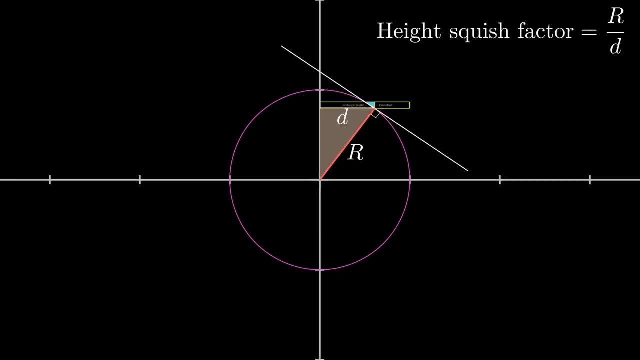 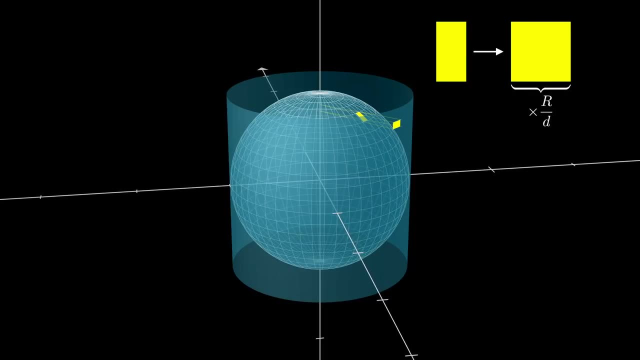 And that's the ratio of this little hypotenuse to the leg on the right side. By the similarity with the big triangle, the ratio of those two sides is again r divided by d. So indeed, as this rectangle gets projected outward, the effect of stretching out the width is perfectly cancelled out by how much that height. 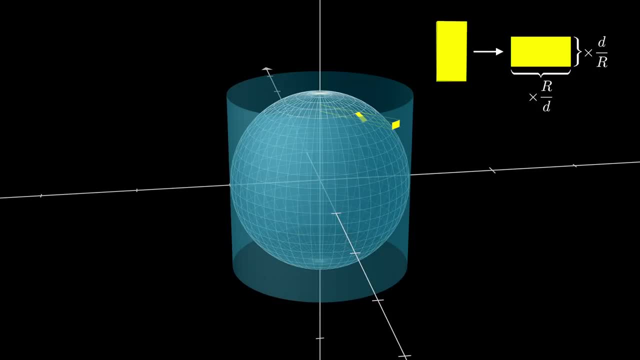 is getting squished due to the slant. As a fun side note, you might notice that it looks like the projected rectangle is a 90 degree rotation of the original. This would not at all be true in general, but, by a lovely coincidence, the way I'm parameterizing the sphere, 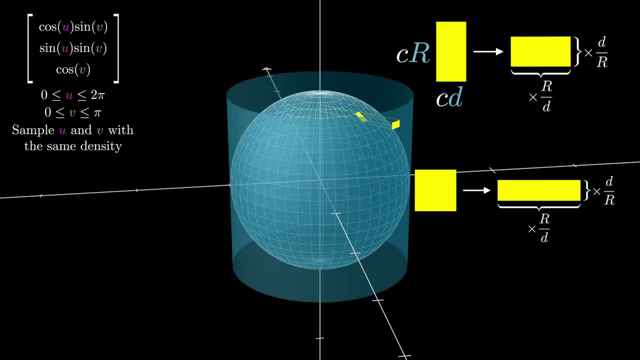 results in rectangles where the ratio of the width to the height starts out as d to r. So for this very specific case, rescaling the width by r over d and rescaling the height by d over r actually does the trick. So, for this very specific case, rescaling the width by r over d and rescaling the height by d over r actually does the trick. So, for this very specific case, rescaling the width by r over d and rescaling the height by d over r actually does the trick. 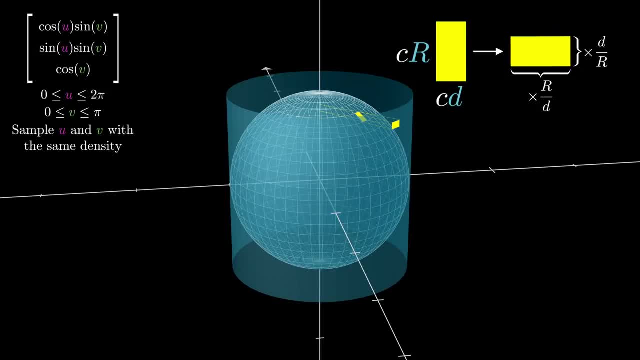 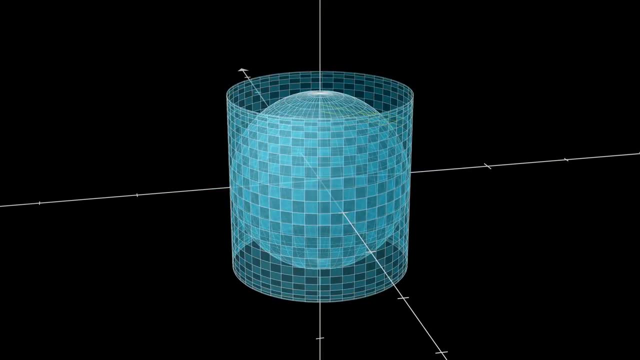 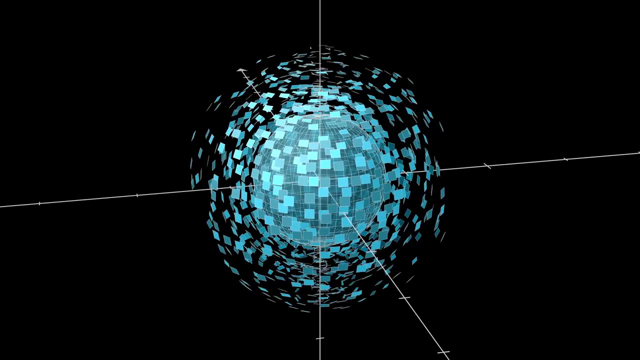 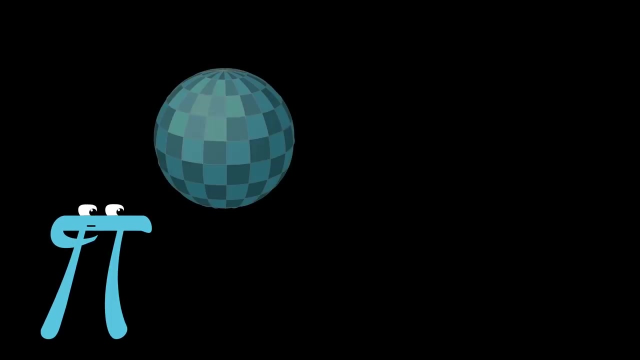 And this lends itself to a rather bizarre way to animate the relation- where, instead of projecting each rectangular piece as if casting a shadow, you can rotate each one of them 90 degrees and then rearrange them all to make the cylinder. Now, if you're really thinking critically, 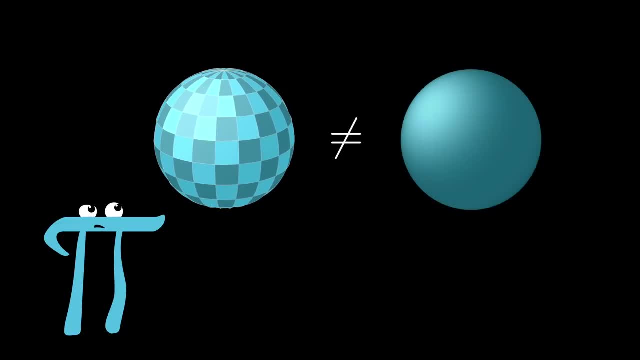 you might still not be satisfied that this shows us what the surface area of the sphere is, because all of these little rectangles only approximate the relevant areas. Well, the idea is that this approximation gets closer and closer to the true value for finer and finer coverings. 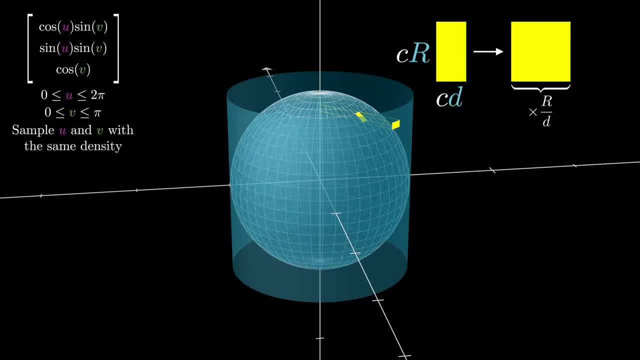 So, for this very specific case, rescaling the width by r over d and rescaling the height by d over r actually does the trick. So, for this very specific case, rescaling the width by r over d and rescaling the height by d over r actually does the trick. 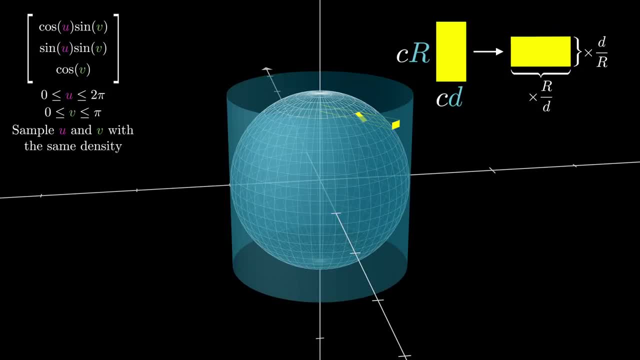 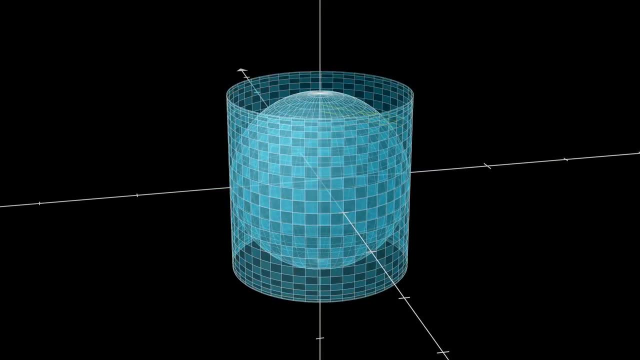 But it does have the effect of a 90 degree rotation, And this lends itself to a rather bizarre way to animate the relation where, instead of projecting each rectangular piece as if casting a shadow, you can rotate each one of them 90 degrees and then rearrange them all to make the cylinder. 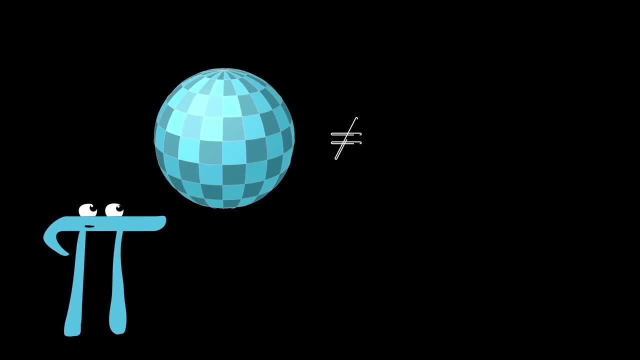 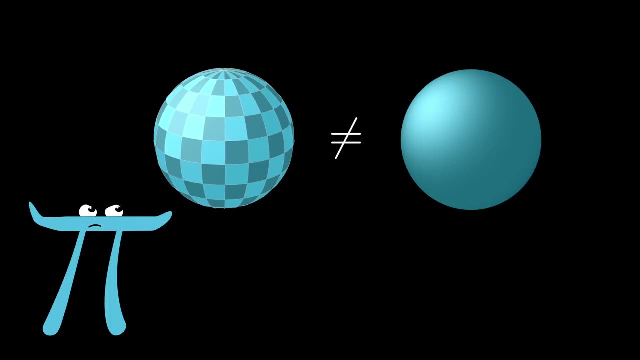 Now, if you're really thinking critically, you might still not be satisfied that this shows us what the surface area of the sphere is, because all of these little rectangles only approximate the relevant areas. Well, the idea is that this approximation gets closer and closer to the true value. 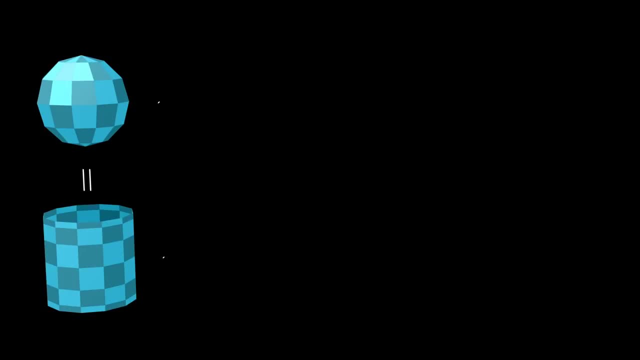 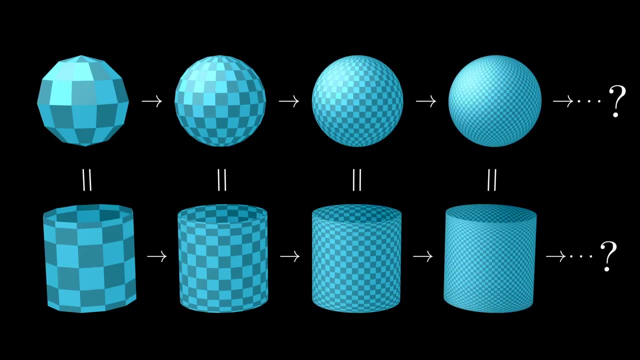 for finer and finer coverings, And since, for any specific covering, the sphere rectangles have the same area as the cylinder rectangles, whatever value each of these two series of approximations are approaching must actually be the same. I mean, as you get really aggressively philosophical about what we even mean by surface area. 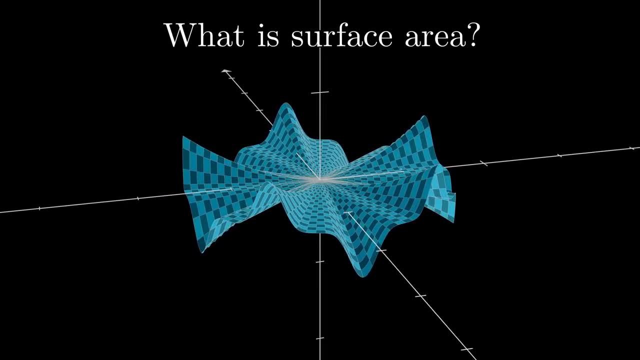 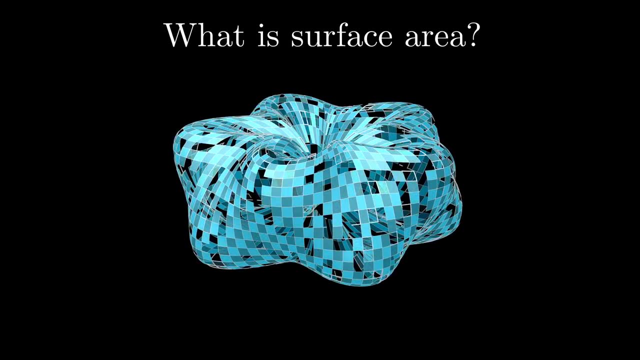 these sorts of rectangular approximations are not just aids in our problem-solving toolbox. They end up serving as a way to rigorously define the idea of area in the context of smooth curved surfaces. This kind of reasoning is essentially calculus, just without any of the jargon. 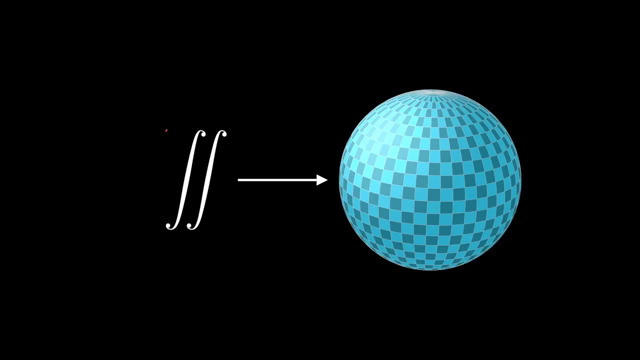 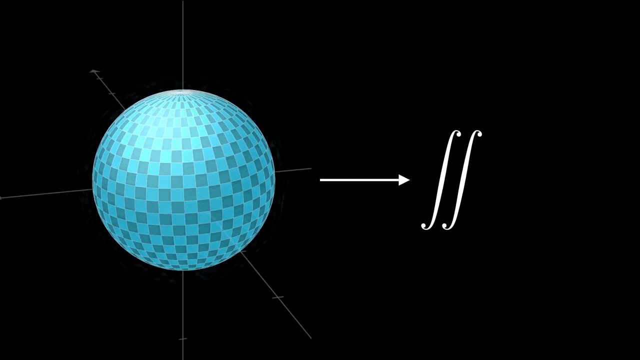 In fact, I think neat geometric arguments like this, which require no background in calculus to understand, can serve as a great way to tee things up for new calculus students so that they have the core ideas already in their head before seeing the definition of surface area. 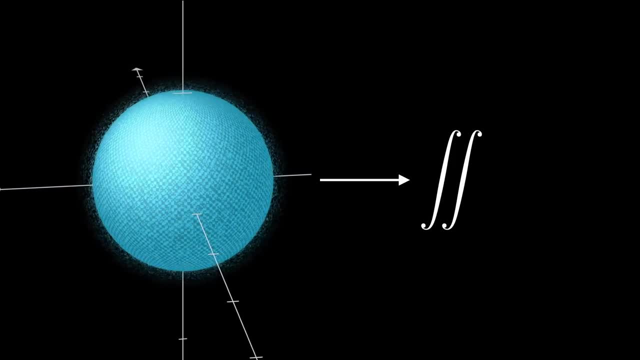 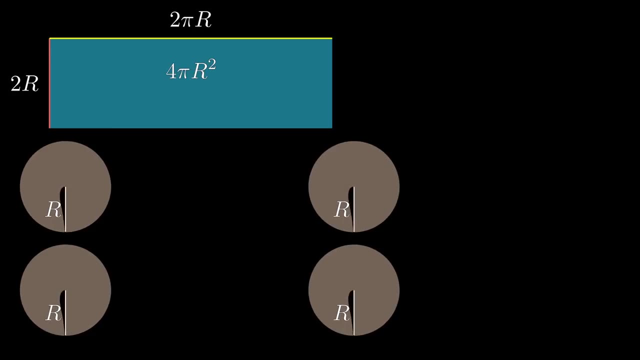 So if you're the kind of person who's just itching to see a direct connection to these four circles, one nice way to do that is to unwrap those circles into triangles. If this is something you haven't seen before, I go into much more detail about why this works in the first video of the calculus series. 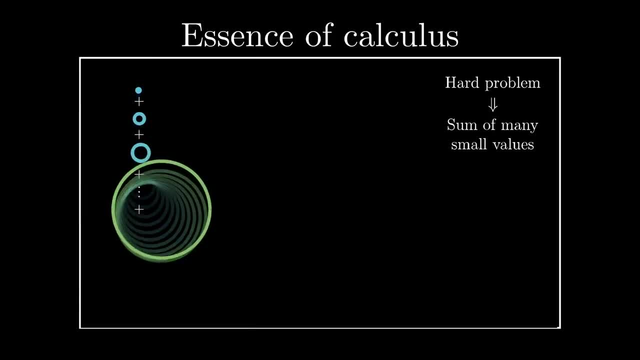 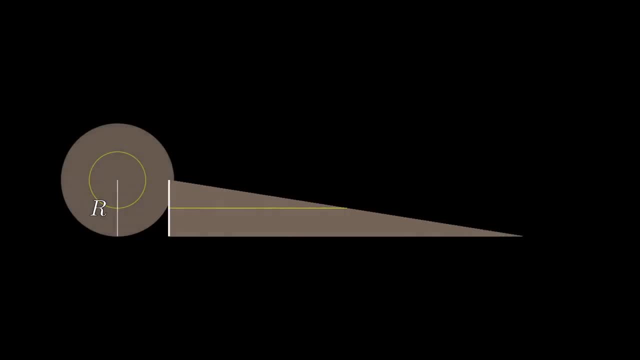 The basic idea is to relate thin concentric rings of the circle with horizontal slices of this triangle, Because if you're not familiar with this, you'll probably have a lot of questions about why this works. But the basic idea is to relate thin concentric rings of the circle with horizontal slices of this triangle. 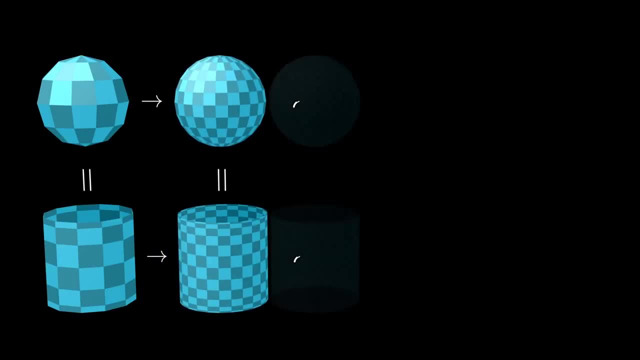 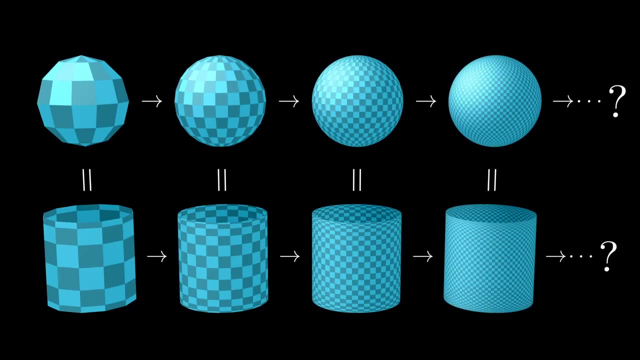 And since, for any specific covering the sphere, rectangles have the same area as the cylinder rectangles, whatever value each of these two series of approximations are approaching must actually be the same. I mean, as you get really aggressively philosophical about what we even mean by surface area. 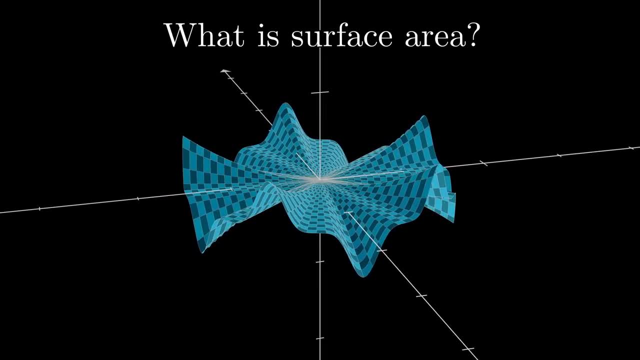 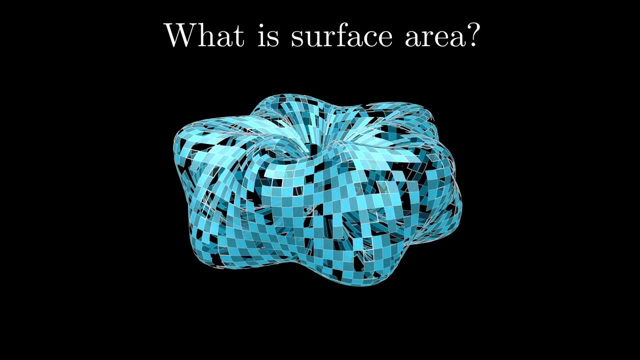 these sorts of rectangular approximations are not just aids in our problem-solving toolbox. they end up serving as a way to rigorously define the idea of area in the context of smooth curved surfaces. This kind of reasoning is essentially calculus, just without any of the jargon. 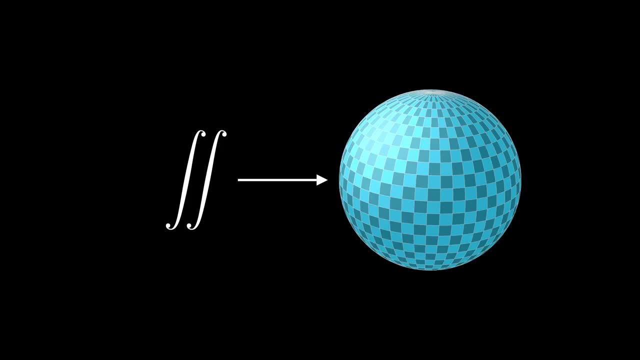 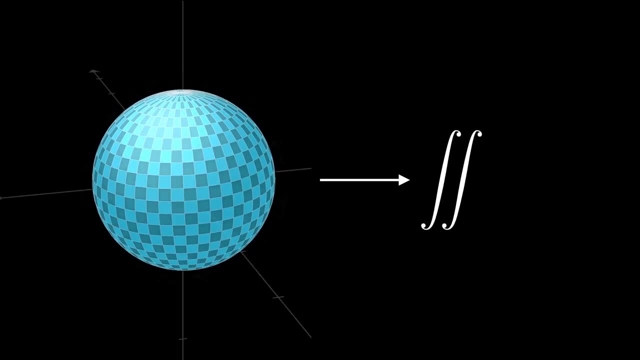 In fact, I think neat geometric arguments like this, which require no background in calculus to understand, can serve as a great way to tee things up for new calculus students so that they have the core ideas already in their head before seeing the definitions which make them precise. 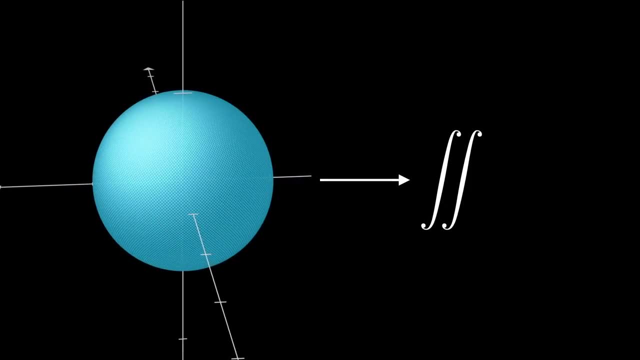 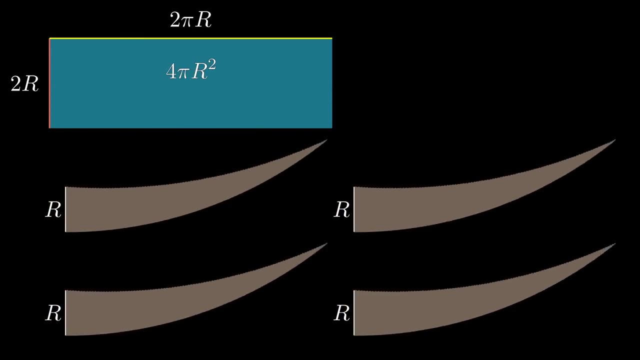 rather than going the other way around. Alright, so, as I said before, if you're the kind of person who's just itching to see a direct connection to these four circles, one nice way to do that is to unwrap those circles into triangles. 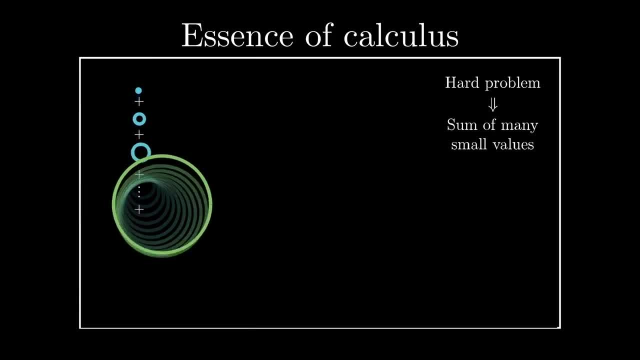 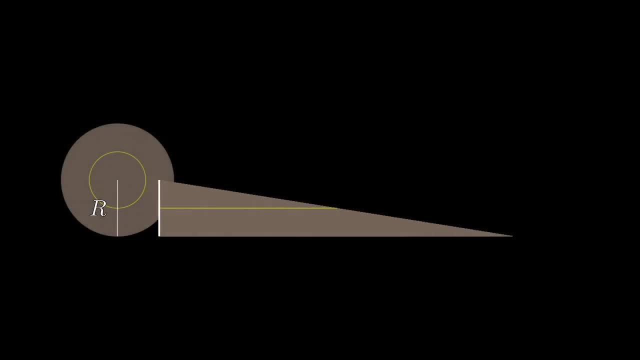 If this is something you haven't seen before, I go into much more detail about why this works in the first video of the calculus series. The basic idea is to relate thin concentric rings of the circle with horizontal slices of this triangle, Because the circumference of each such ring increases linearly in proportion to the radius. 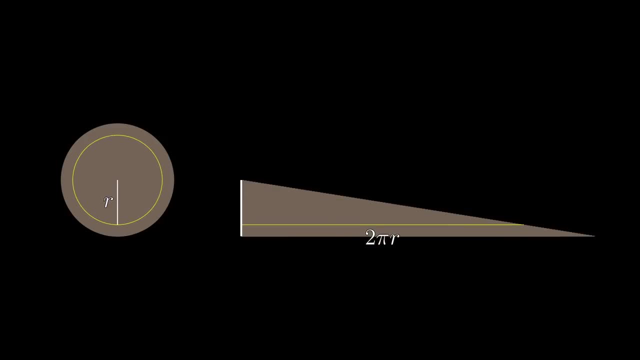 always 2 pi times that radius. when you unwrap them all and line them up like this, their ends will form a straight line, as opposed to some other curved shape, which gives us a triangle with base 2 pi r and height r. 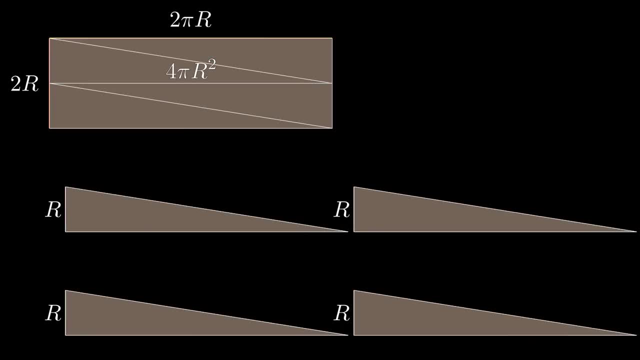 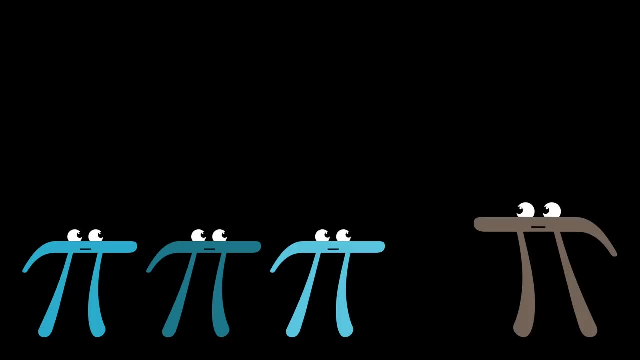 And four of these unwrapped circles fit perfectly into our rectangle, which is, in some sense, an unwrapped version of the sphere's surface. Now, that's a lot of work, isn't it? So let's get started. That's pretty satisfying. 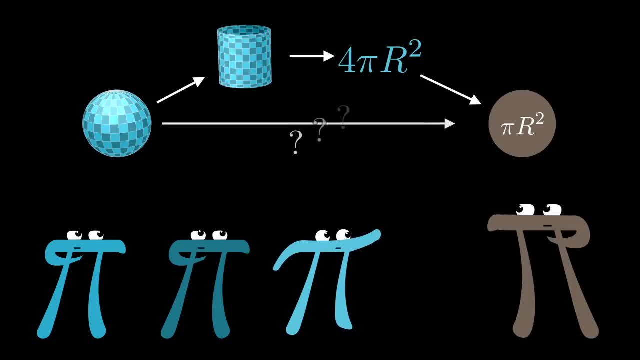 But you might nevertheless be wondering if there's some way to relate this sphere directly to a circle with the same radius, rather than going through this intermediary of a cylinder. I do have a proof for you to this effect, leveraging a little trigonometry. 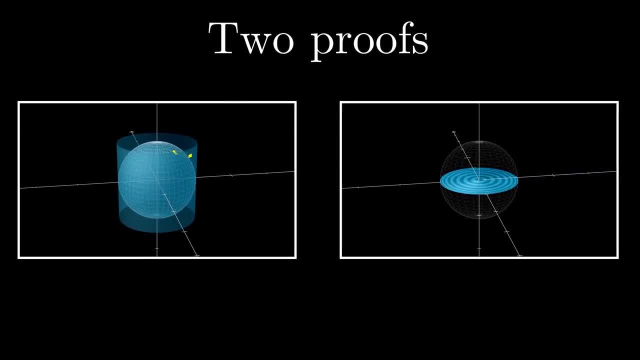 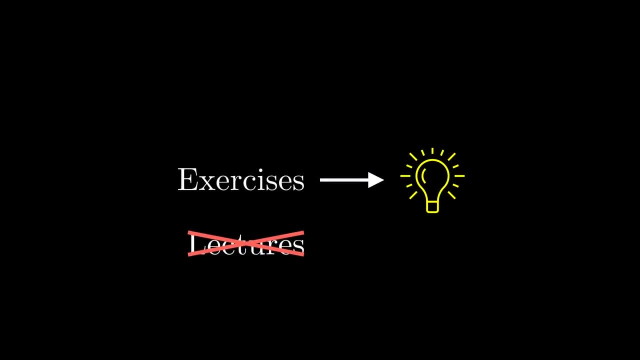 though I have to admit, I still think the comparison to the cylinder wins out on raw elegance. Now, I'm a big believer that the best way to really learn math is to do problems for yourself, which is a bit hypocritical coming from a channel essentially consisting of lectures. 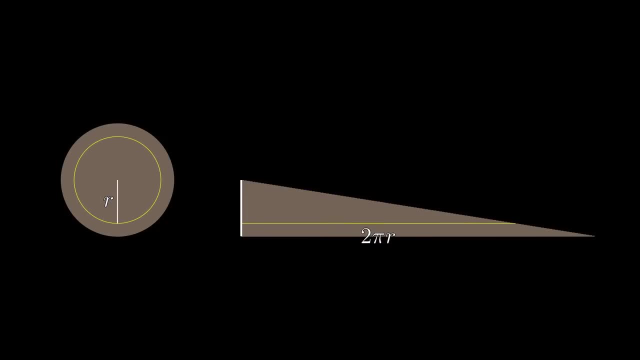 Because the circumference of each such ring increases linearly in proportion to the radius, always 2 pi times that radius. when you unwrap them all and line them up like this, their ends will form a straight line, as opposed to some other curved shape. 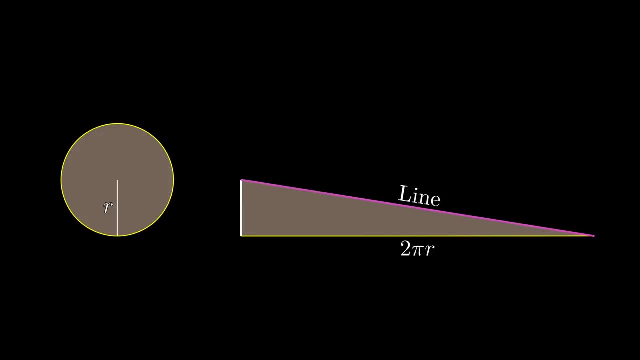 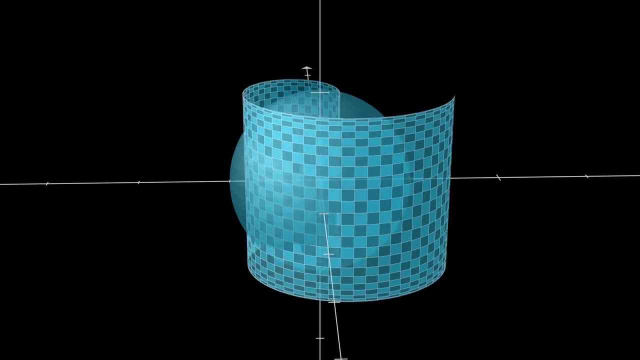 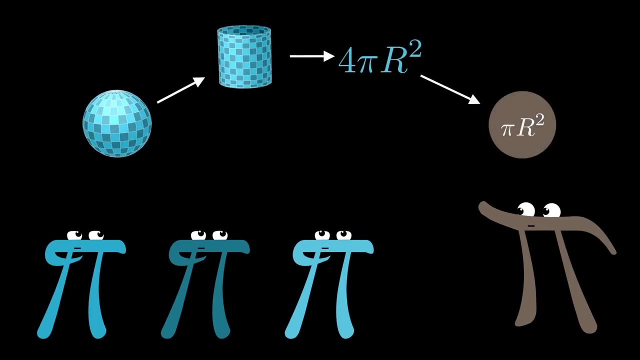 which gives us a triangle with base 2, pi r and height r, And four of these unwrapped circles fit perfectly into our rectangle, which is in some sense, an unwrapped version of the sphere's surface. Now, that's pretty satisfying, but you might nevertheless be wondering if there's some way to relate this sphere 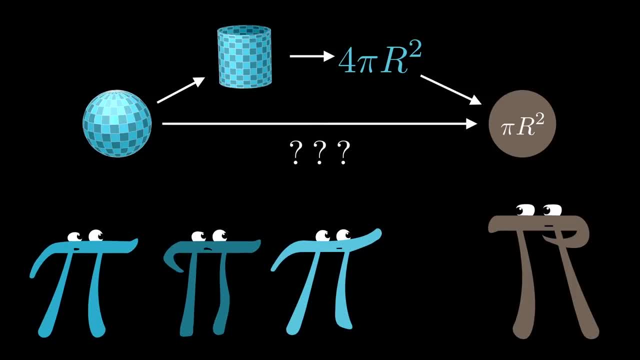 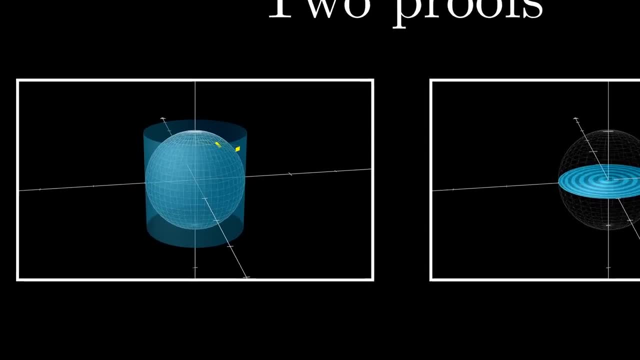 directly to a circle with the same radius, rather than going through this intermediary of a cylinder. I do have a proof for you to this effect, leveraging a little trigonometry, though I have to admit I still think the comparison to the cylinder wins out on raw elegance. 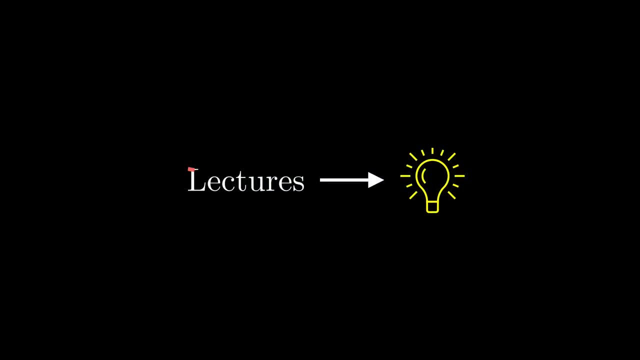 Now, I'm a big believer that the best way to really learn math is to do problems for yourself, which is a bit hypocritical coming from a channel essentially consisting of lectures, So I'm going to try something a little different here and present the proof as a heavily guided sequence of exercises. 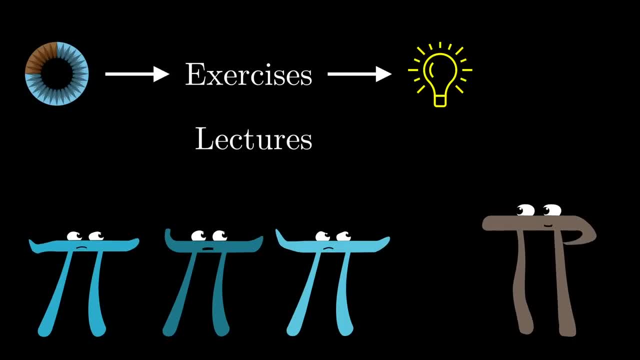 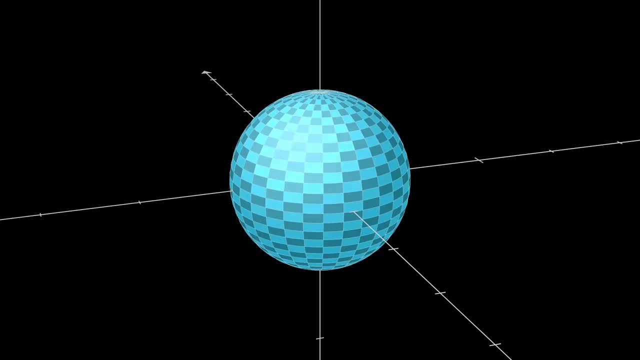 Yes, I know that's less fun and it means you have to pull out some paper to do a little work, but I guarantee you will get more out of it this way At a high level. the approach will be to cut the sphere into many thin rings parallel to the xy-plane. 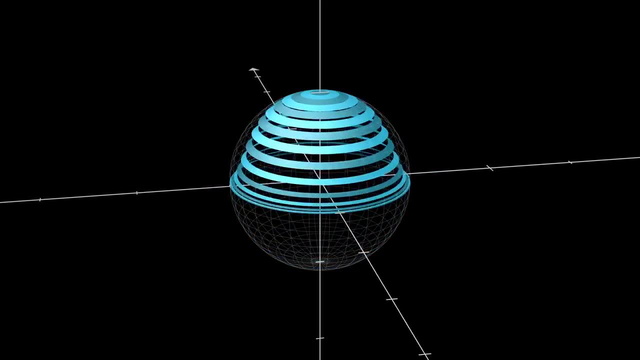 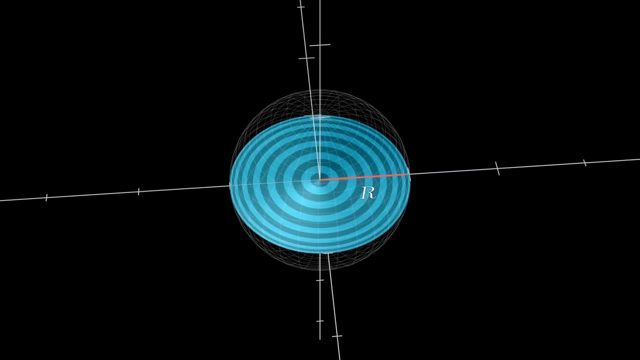 and to compare the area of these rings to the area of their shadows on the xy-plane. All of the shadows of the rings from, say, the northern hemisphere make up a circle with the same radius as the sphere right. Well, the main idea will be to show a correspondence between these ring shadows. 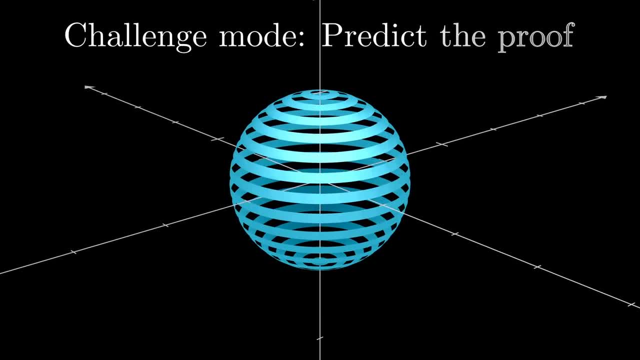 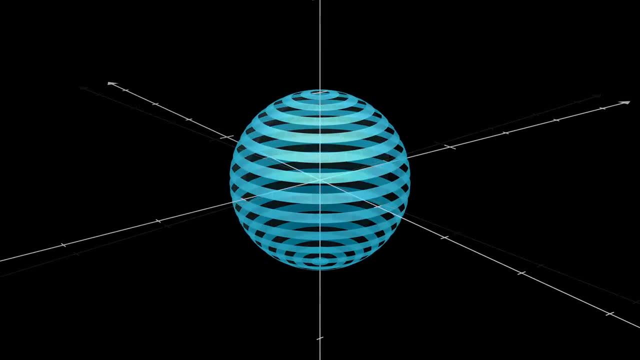 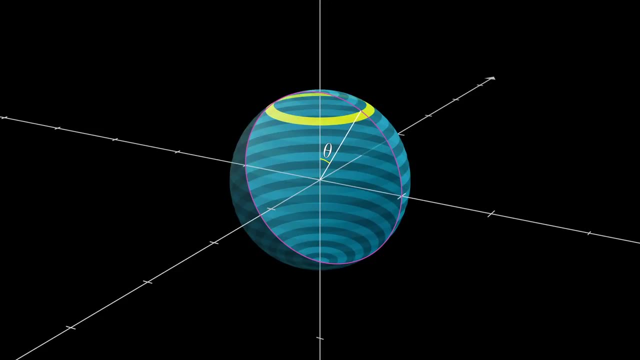 and every second ring on the sphere. Challenge mode here is to pause now and see if you can predict how that comparison might go. Let's label each one of these rings based on the angle theta between a line from the sphere's center to that ring and the z-axis. 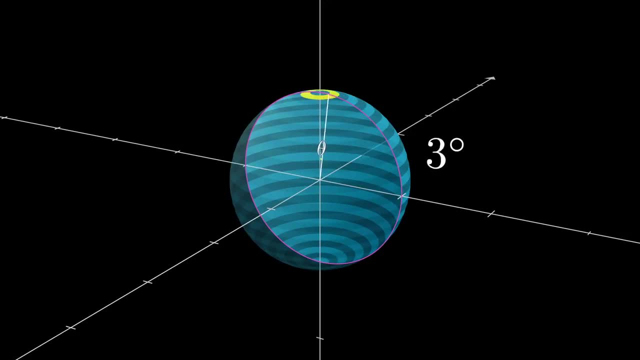 So theta ranges from zero at the north pole all the way up to 180 degrees at the south pole, which is to say from zero to pi radians. And let's call the change in the angle from one ring to the next d theta, which means the thickness. 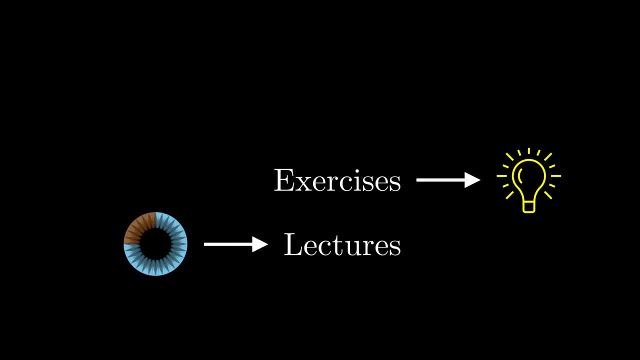 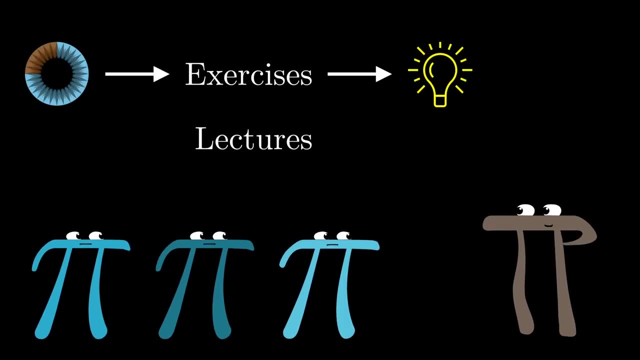 so I'm going to try something else. I'm going to try something a little different here and present the proof as a heavily guided sequence of exercises. Yes, I know that's less fun and it means you have to pull out some paper to do a little work. 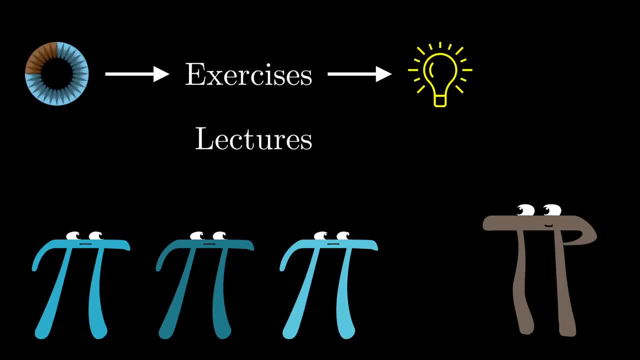 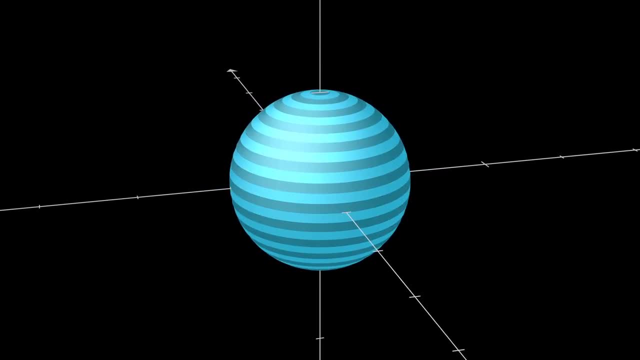 but I guarantee you will get more out of it this way At a high level. the approach will be to cut the sphere into many thin rings parallel to the xy-plane and to compare the area of these rings to the area of their shadows on the xy-plane. 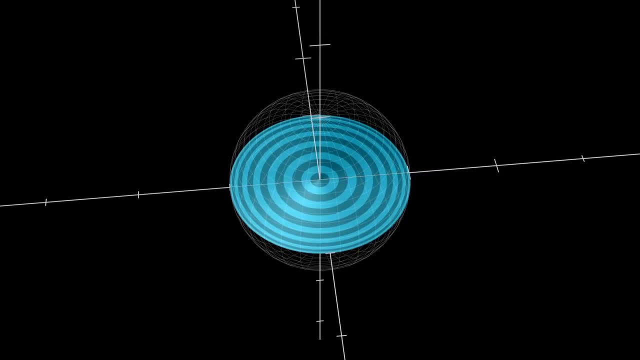 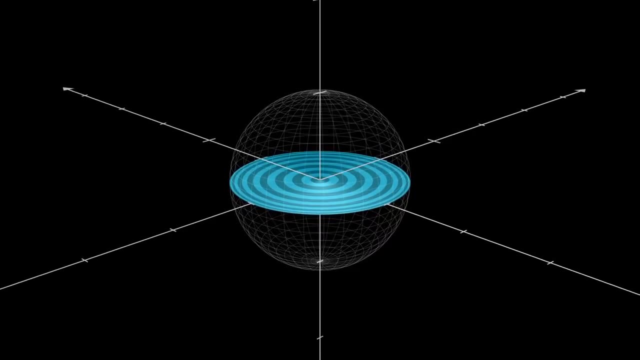 All of the shadows of the rings from, say, the northern hemisphere make up the xy-plane. They make up a circle with the same radius as the sphere, right? Well, the main idea will be to show a correspondence between these ring shadows. 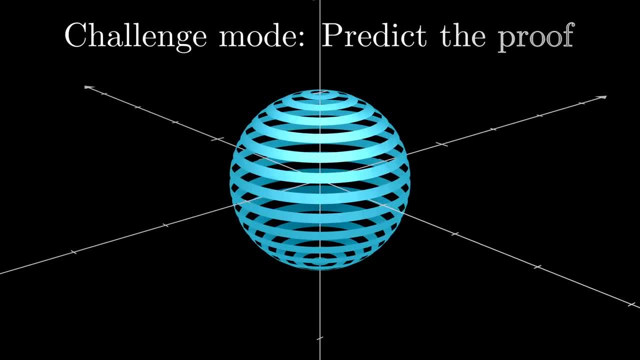 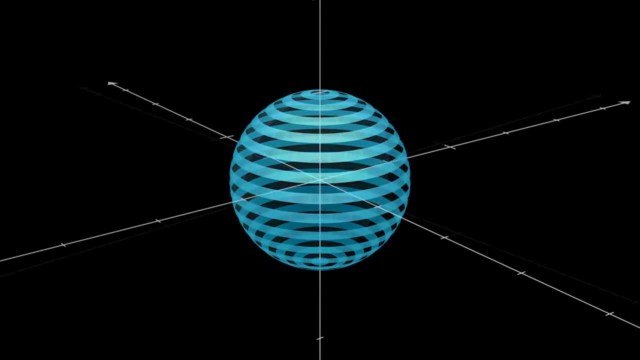 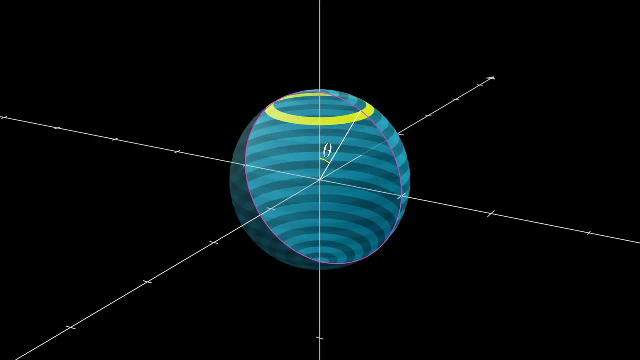 and every second ring on the sphere. Challenge mode here is to pause now and see if you can predict how that comparison might go. Let's label each one of these rings based on the angle theta between a line from the sphere's center to that ring and the z-axis. 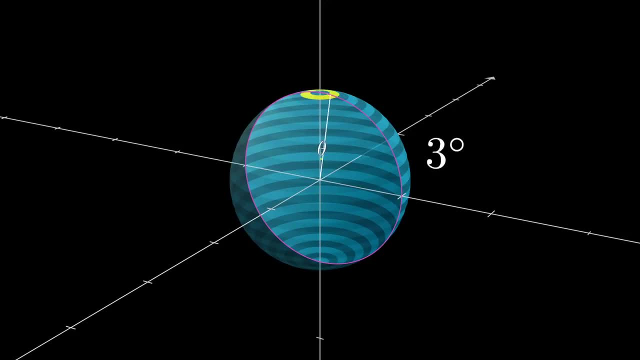 So theta ranges from zero at the north pole all the way up to 180 degrees at the south pole, which is to say from zero to pi radians, And let's call the change in the angle from one ring to the next d theta. 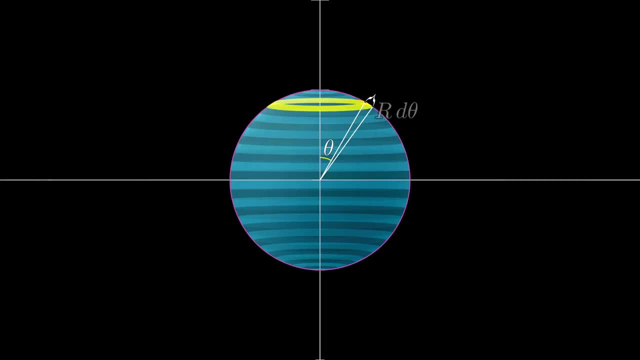 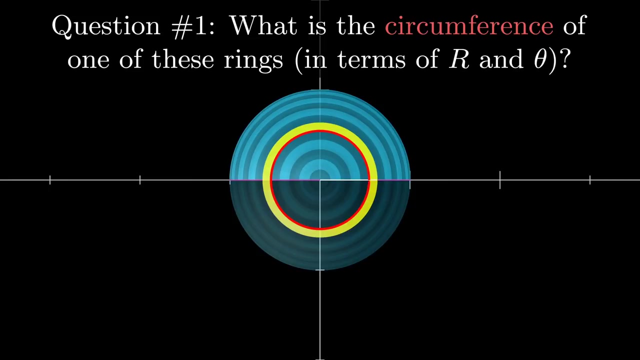 which means the thickness of those rings will be the radius, r, times, d, theta. Alright, structured exercise time. We'll ease in with a warm up. Question number one: what is the circumference of this ring, say at the inner edge, in terms of r and theta? 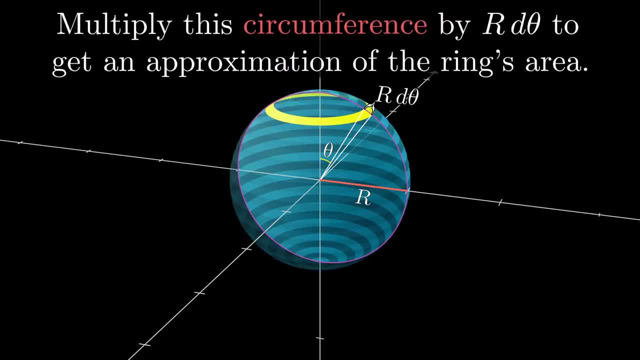 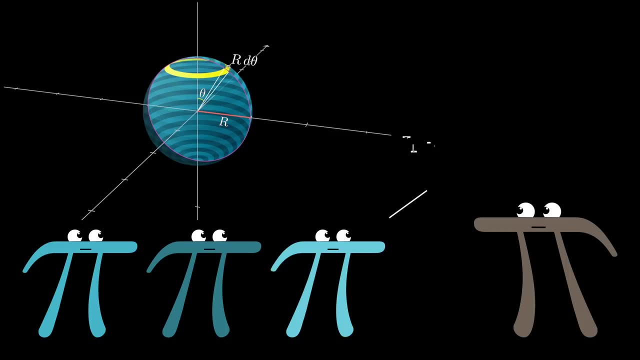 Once you have that, go ahead and multiply the answer by the thickness r times d theta to get an approximation for the ring's area, An approximation that will get better and better as you chop up the sphere more and more finely And at this point, if you know your calculus, you could integrate. 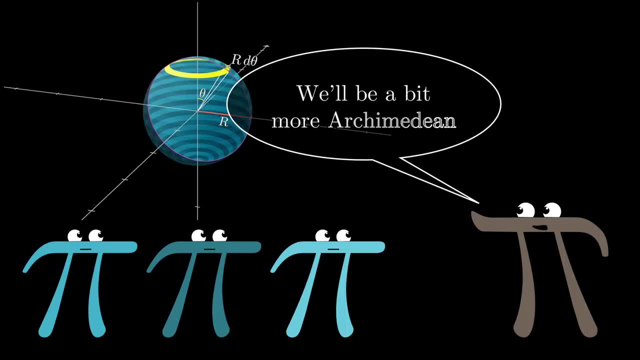 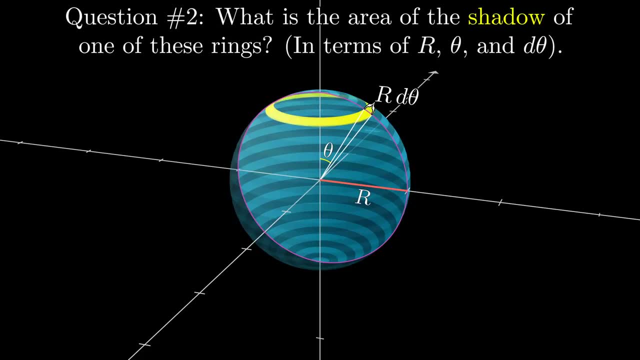 But our goal is not just to find the answer, it's to feel the connection between the sphere and its shadow. So question number two: What is the area of the sphere? Well, the area of the sphere is the shadow of one of these rings on the x-y plane. 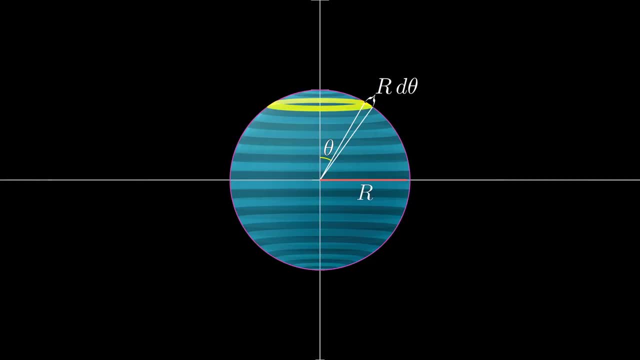 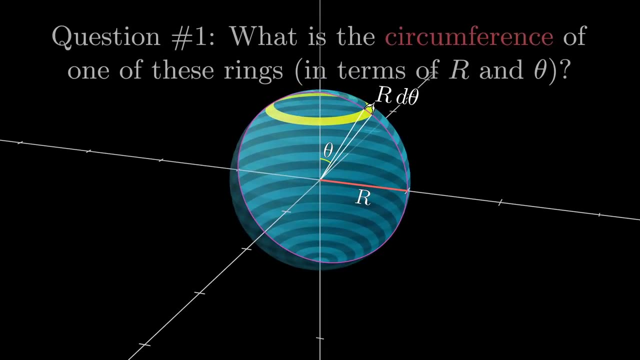 of those rings will be the radius, r, times, d, theta. All right, structured exercise time. We'll ease in with a warmup. Question, number one: what is the circumference of this ring, say at the inner edge, in terms of r and theta? 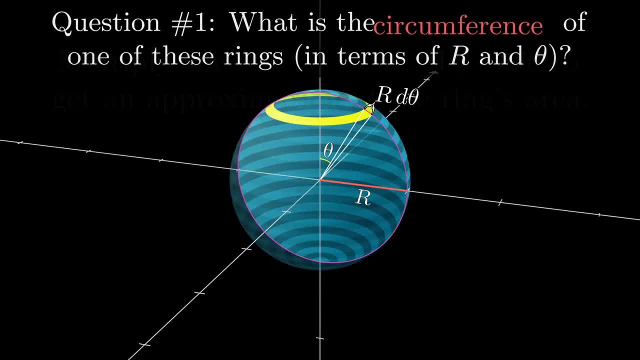 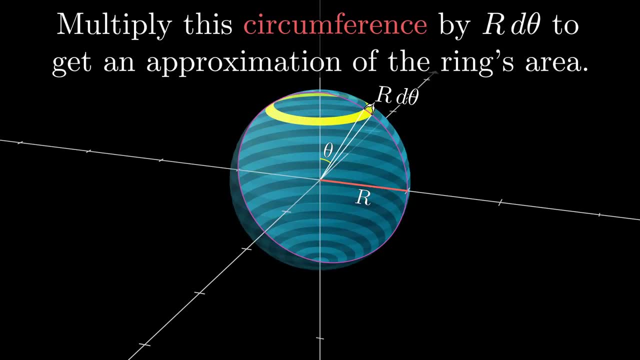 Once you have that, go ahead and multiply the answer by the thickness r times d theta to get an approximation for the ring's area, an approximation that will get better and better as you chop up the sphere more and more finely. And at this point, if you know your calculus, 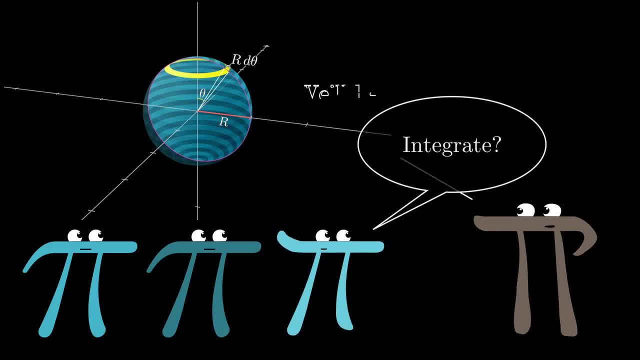 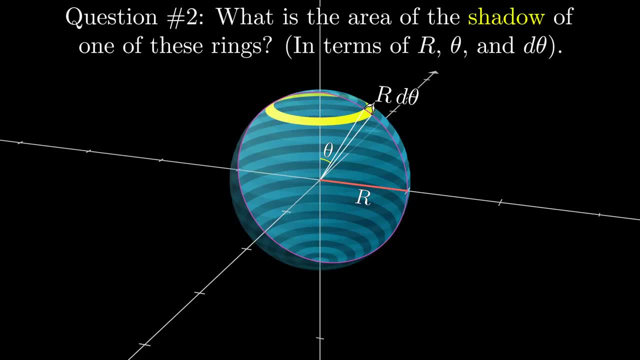 you could integrate. but our goal is not just to find the answer, it's to feel the connection between the sphere and its shadow. So question number two: what is the circumference of one of these rings on the x- y plane? What is the area of the shadow of one of these rings? 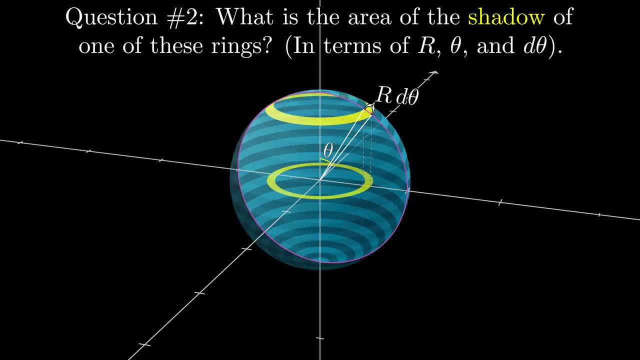 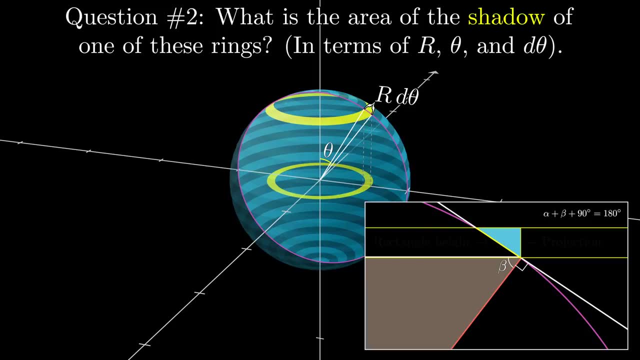 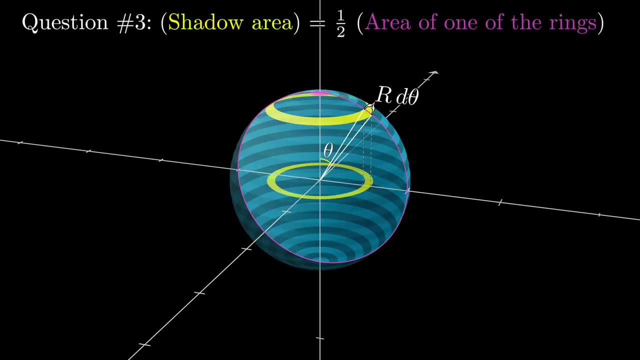 on the x? y plane, Again expressed in terms of r? theta and d? theta, And for this one it might be helpful to think back to that tiny little right triangle we were talking about earlier. Question number three, and this is really the heart of it, 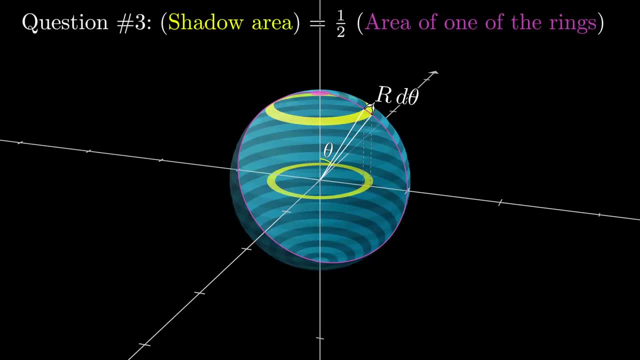 each one of these rings' shadows has precisely half the area of one of the rings on the sphere. It's not just one little theta straight above it, but another one. The question is, which one? As a hint, you might want to reference some trig identities. 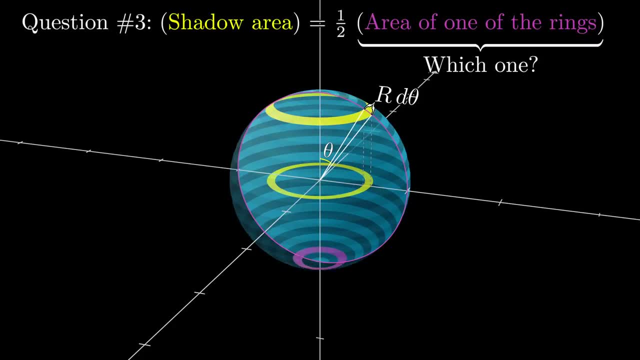 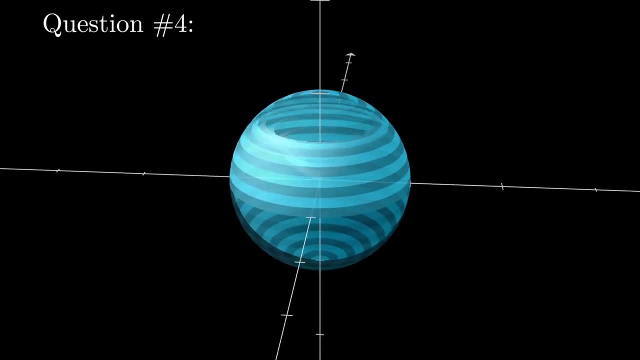 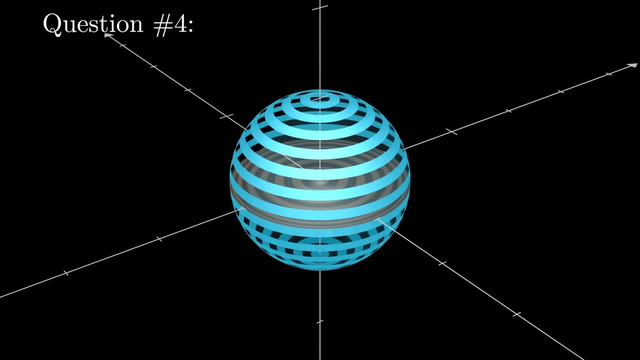 for this one, Question number four. I said at the outset that there's a correspondence between all of the shadows from the northern hemisphere, which make up a circle with radius r, and every second ring on the sphere. Use your answer to the last question to spell out what exactly the ring is on the sphere. 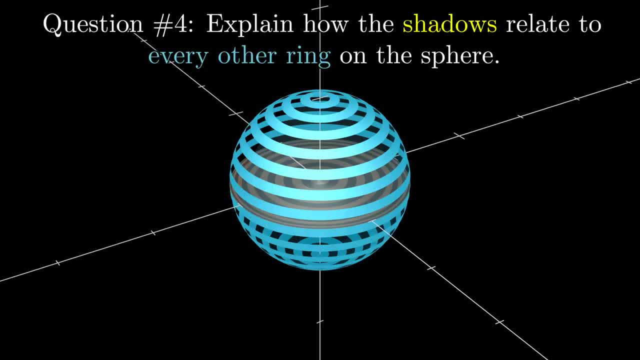 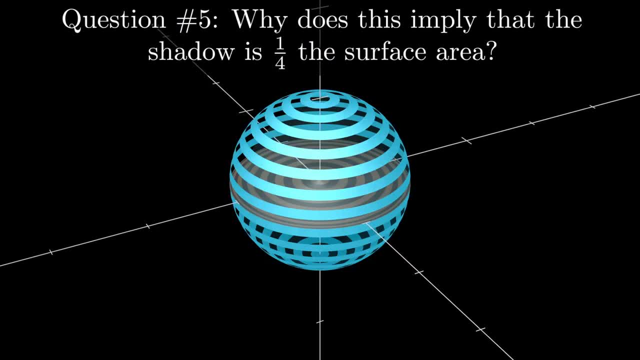 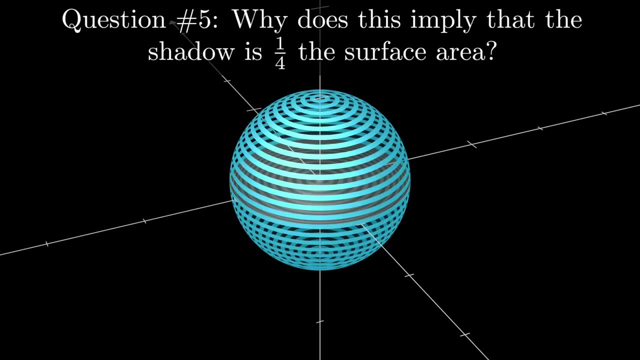 And for question five, bring it on home. Why does this imply that the area of the circle is exactly one-fourth the surface area of the sphere, particularly as we consider thinner and thinner rings? If you want answers or hints, I'm quite sure that people in comments and on Reddit 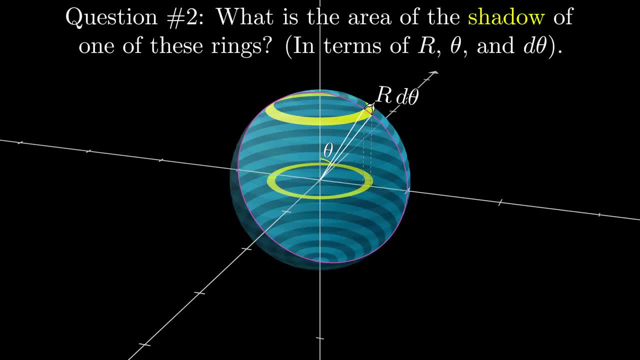 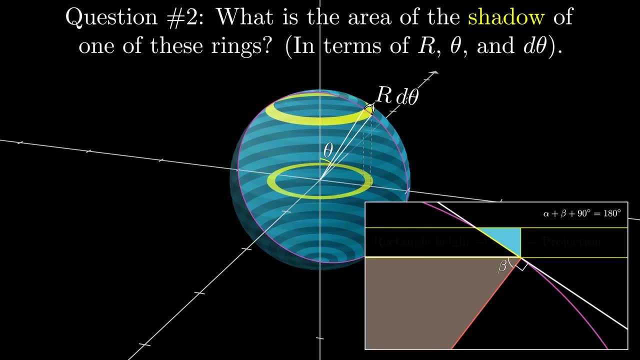 Again expressed in terms of r? theta and d theta, And for this one it might be helpful to think back to that tiny little right triangle we were talking about earlier. Question number three, and this is really the heart of it.